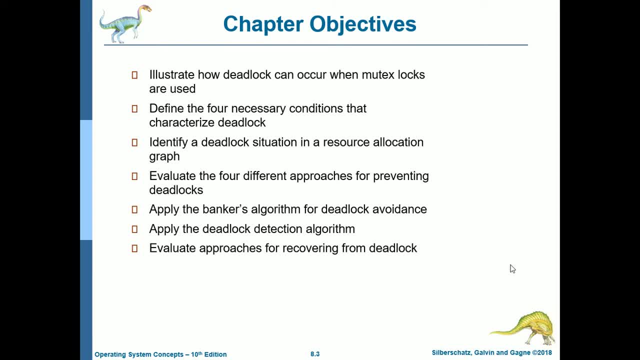 deadlock can occur when mutex locks are used. Define the four necessary conditions that correct deadlock can occur when mutex locks are used. Define the four necessary conditions that characterize deadlock. Identify a deadlock situation in the resource allocation graph. Evaluate the four different approaches for preventing deadlocks. Apply the banker's. 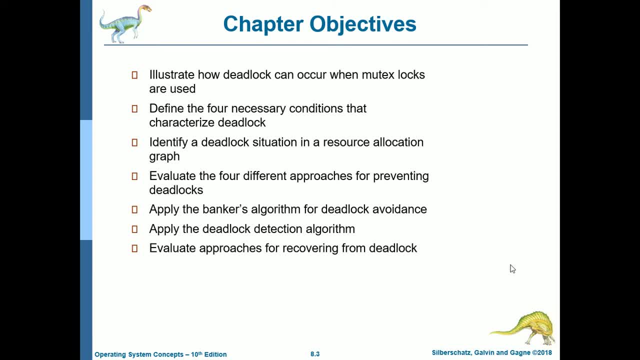 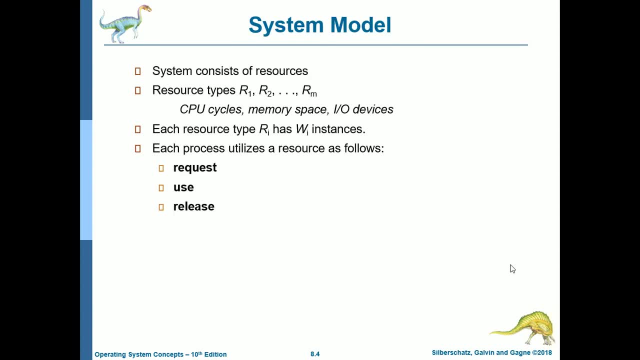 algorithm for deadlock avoidance, Apply the deadlock detection algorithm And evaluate approaches for recovering from deadlock. So the system model, So system consists of resources, So these are resource types, So it has a notation of resources. And then the fourth is illustrate how deadlock can occur when mutex locks are used. 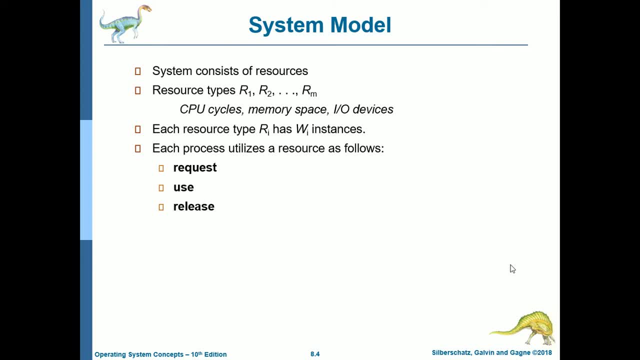 R1,, R2, until Rm. So the example of resource types that is available in a computer system are the CPU cycles, memory space and input-output devices. So for these resource types So Ri has wi instances. Example in a computer system we have i0 devices. 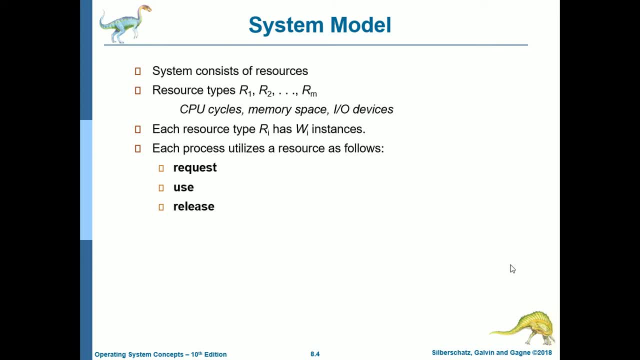 or the number of existing i0 devices is equal to five. So that's already an example of the wi. And then the seventh is illustrate how deadlock can occur when mutex locks are used. To samples. it should be written: and通: r1 to r4 and r5. 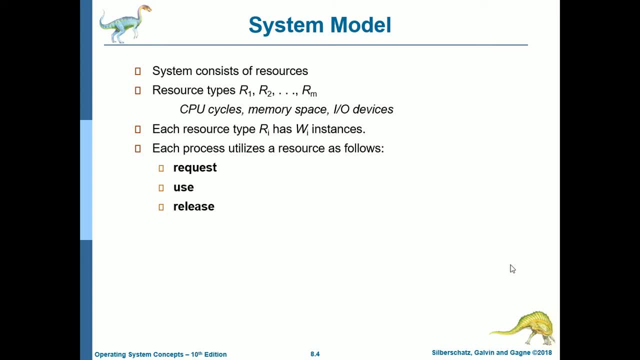 So that's already an example of the W-sub-I instances. So each process utilizes a resource as follows. So for a process to use a certain type of resource, it should request for that resource And after the request is granted for that resource, the process can already use that particular resource type. 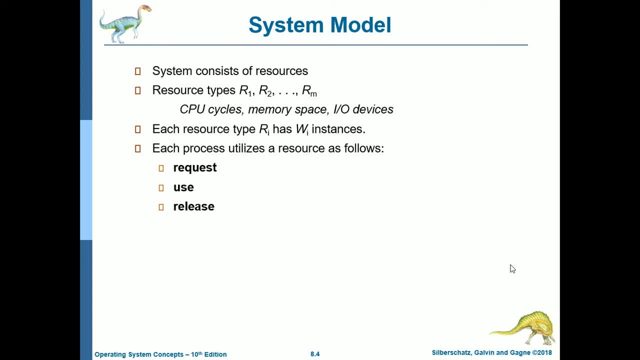 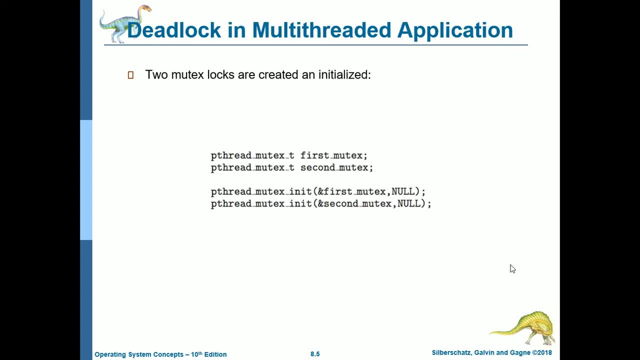 And then, after the process is executed, it should release the resources that it's allocated to that particular process. So deadlock in a multi-threaded application. So, assuming that we have two mutex locks, that is created and initialized. So this is the two mutex locks and this is their initializing command. 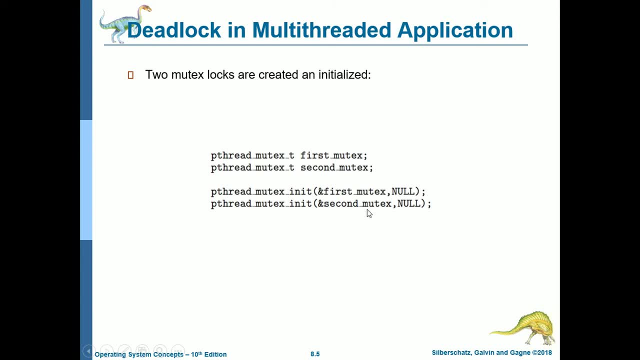 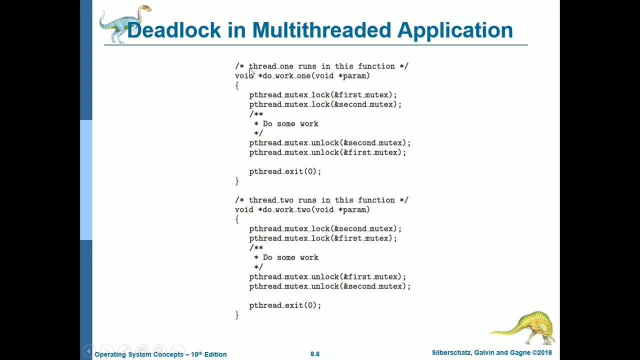 So for the first mutex and the second Mutex lock, And then we have a code here in which let's read the comment: So thread underscore one runs in this function. And then we have another code for thread two runs in this function. 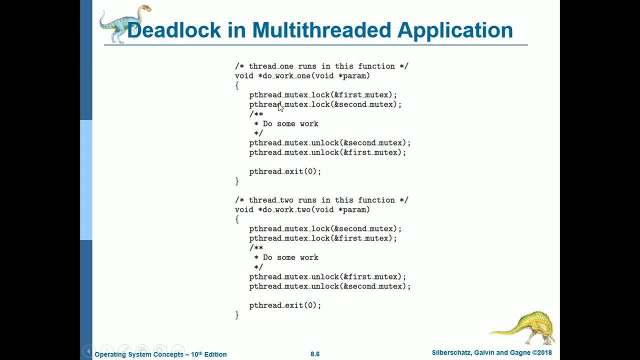 As we can see that the two threads has access to both of the mutex locks, So we have first and second mutex locks. So actually with this example there is deadlock. So what if thread One has access for has already acquired the first mutex locks and thread two acquired the second mutex lock? 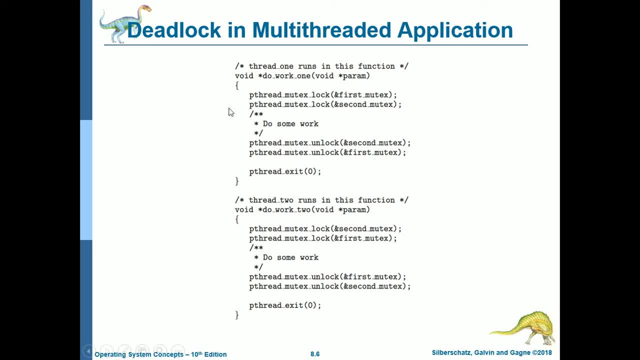 But both of the threads need these two mutex locks to execute or it will be used by the thread. So because of that situation, the thread one acquires the first mutex And then the thread number two acquires the second mutex, And then they both need those mutex locks. 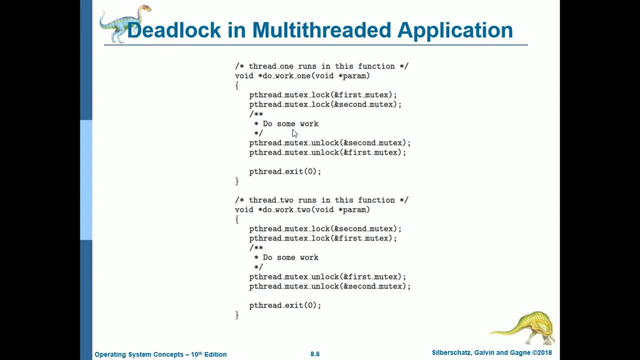 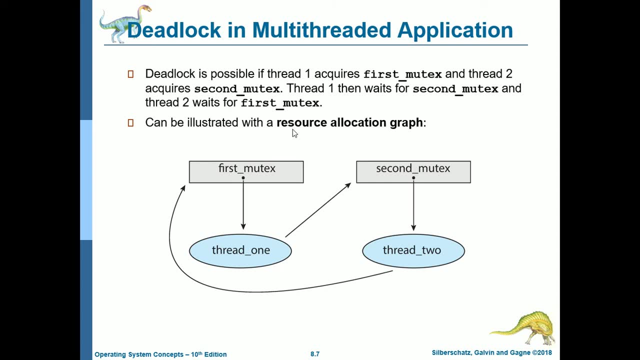 So this is already a classic example of a deadlock. So deadlock is possible, as I've said, if thread one acquires first underscore mutex and thread two acquires second underscore mutex. as I've said, Thread one then waits for the second underscore mutex and thread two waits for first underscore mutex. 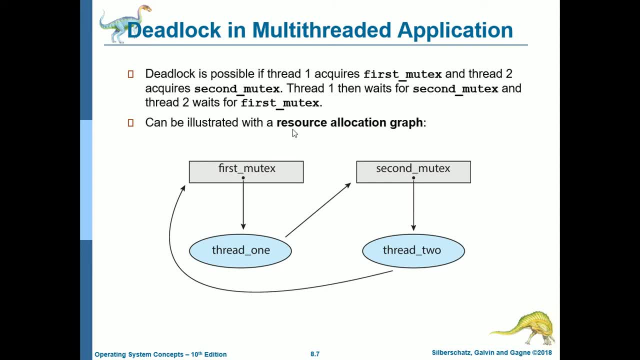 As I've said, with the example of two students And then the resource: they're going to have A drawing session and then you have a pencil and paper. And then what if student A has acquired the pencil and the student B has acquired the paper? 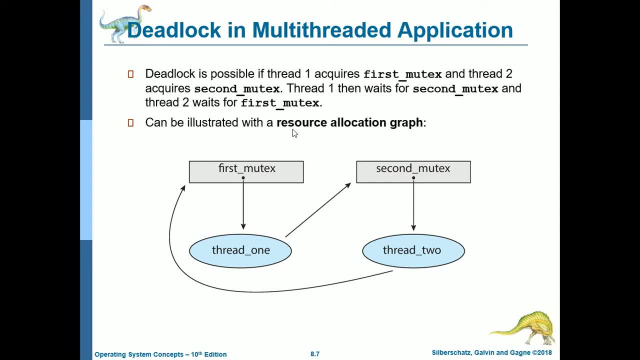 So there is deadlock because no one will give in. For example, since student A already has the pencil, he or she will wait for the paper, while the student B- since the student B has already acquired the paper, he or she will wait for the release of the pencil. 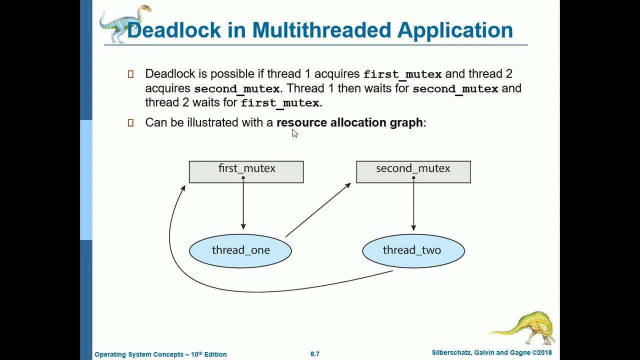 So this example of a deadlock, so this is very simple- two threads and then two resources. So it can be illustrated with a resource allocation graph. So this is the illustration: for the first mutex, It is already acquired by thread number one. And then the second mutex is already acquired by thread number two. 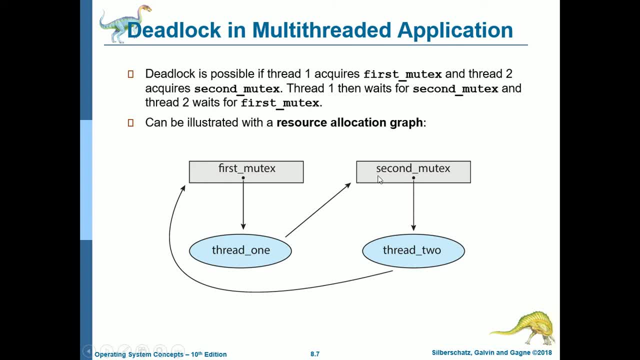 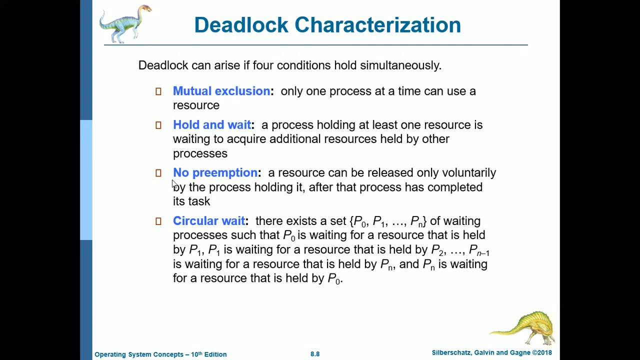 And thread number one waits for the Release of the second mutex, while the thread two also waits for the release of the first mutex. So that is already a deadlock. Both are waiting. who will release the particular resource? Okay, so deadlock characterization. So deadlock can arise if four conditions hold simultaneously. 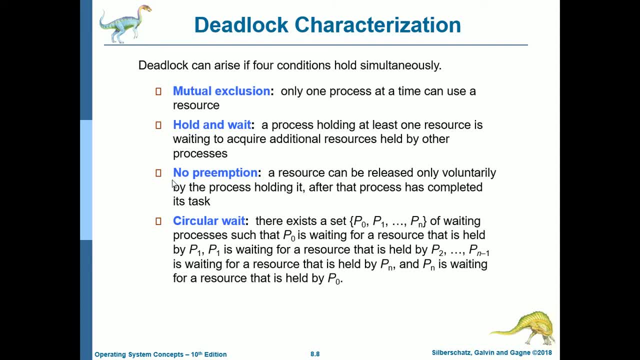 So these are the four conditions and it is end. All of them should occur all at the same time. So first is we have the mutual exclusion, So only one process at a time can use a resource, And then we also have hold and wait. 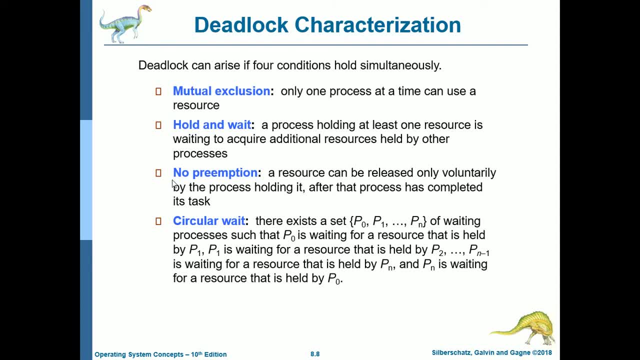 So for the number of process using the resource. so a process holding at least one resource is waiting to acquire additional resources held by other processes. It means that at least one one of the process is waiting. For example, the process has already acquired its resources, of course, but it's not yet enough. 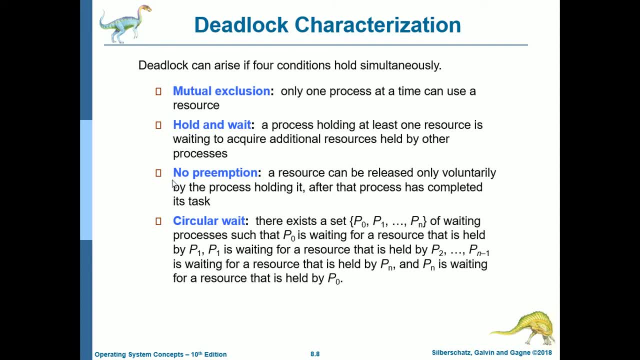 And it's waiting to acquire additional resources held by other processes. And then next is we have the no-preemption: A resource can be released only voluntarily by the process holding it after that process has completed its task. So it means that the release of the resources will only be possible if the process holding that resources already finished its execution. 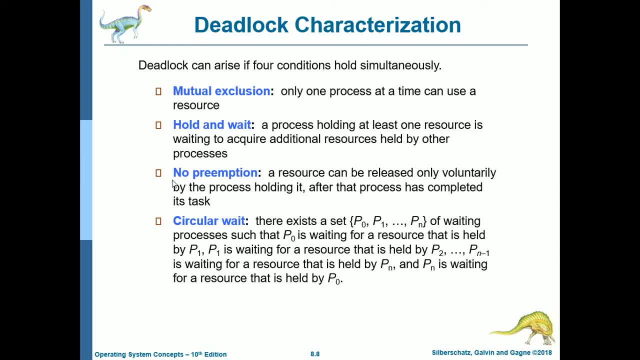 And then we also have the circular wait. there exists a set of- from P0 to Pn- of waiting processes, such that P0 is waiting for a resource that is held by P1, while P1 is waiting for a resource that is held by P2, and then that will. 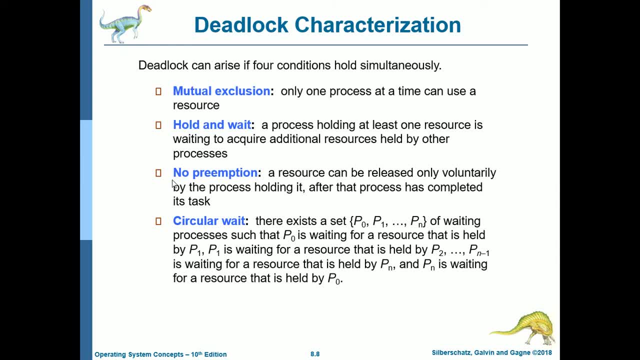 go on until Pn-1, and then Pn-1 is waiting for a resource that is held by Pn, and Pn is waiting for a resource that is held by P0. So these processes are waiting in a cycle, So as you can. 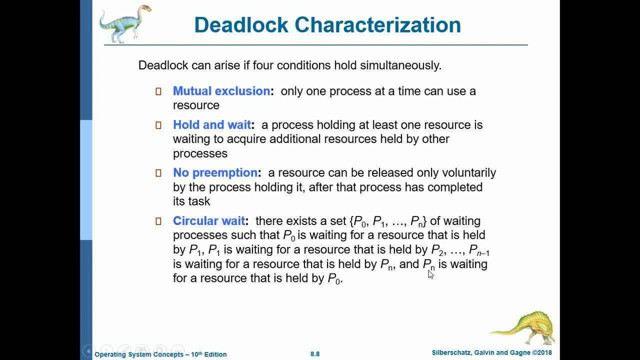 see the maximum number of processes. for example, we have Pn is also waiting for a resource that is held by P0.. So actually the fourth condition: this will really determine if there is a deadlock because of the circular wait. 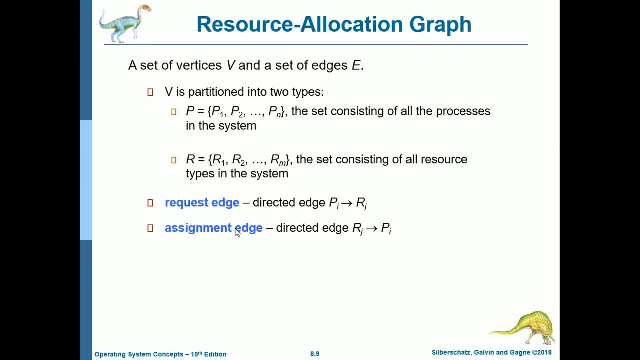 So we have a process that is held by P0.. So we have a process that is held by P0.. So we have a resource allocation graph. So this shows graphically to easily understand if there is a deadlock or not in a situation of processes requesting for a particular resource. So 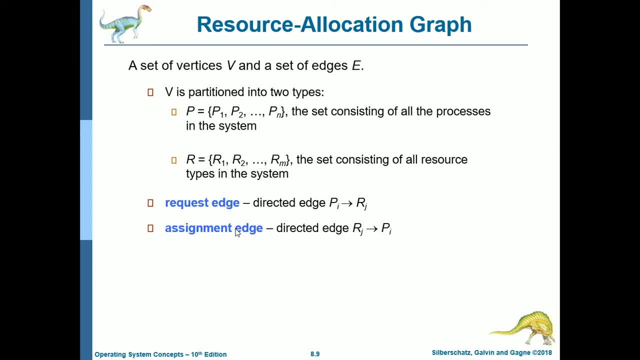 a resource allocation graph is a set of vertices- V- and a set of edges- E. So V is partitioned into two types. So we have P, from P1 to Pn. These are the set consisting of all the processes in the system, And then we have R, from R1 to Rm, as its notation, The set consisting of all resource. 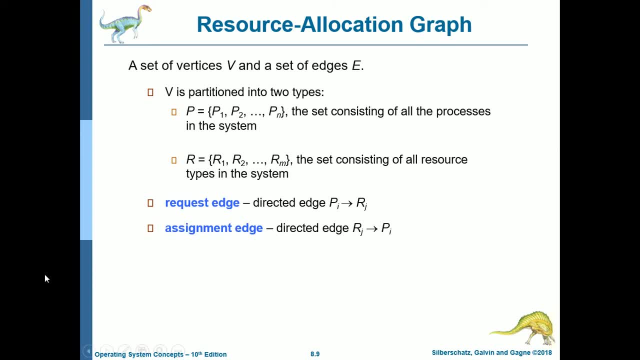 types in the system. So we have two edges. So request edge is a directed edge from Pi going to P going to R. If the arrow is from P going to R, it is a request edge, meaning that the process has not yet acquired that particular resource and requests for that particular resource. So we have 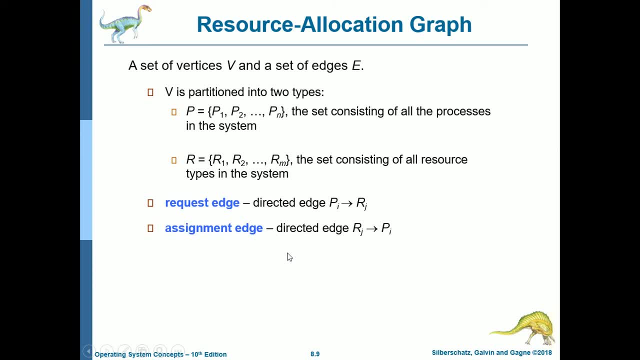 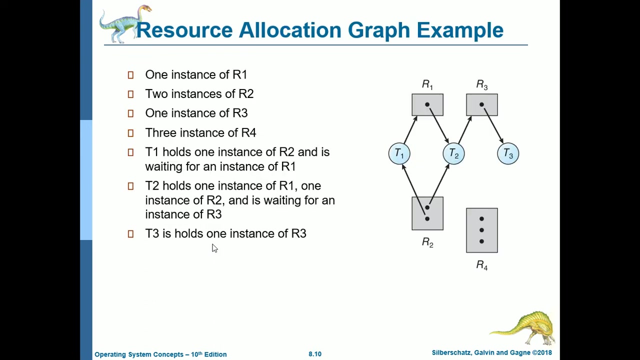 an example of a resource allocation graph. So from the right of our slide we have a resource allocation graph. So we have. so let's just enumerate. So one instance of R1. So this is the resource R1, only one resource for R1. And then two instances of R2.. So this is R2.. It has two. 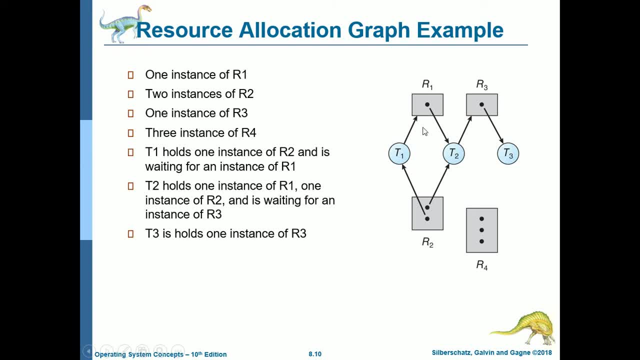 instances And then one instance of R3.. So one instance only And then three instances of R4.. So as you can see, no, okay, this T here is thread. Okay, sometimes it is process and sometimes it can be a thread. So, 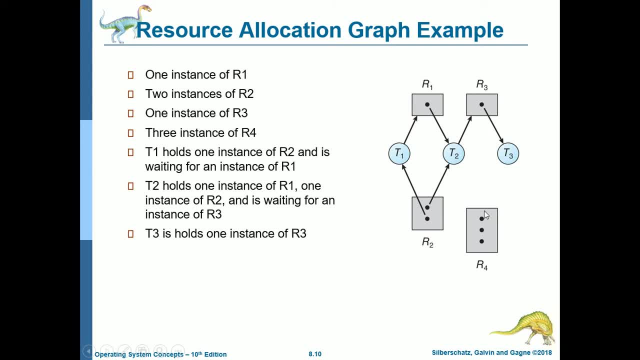 that's why it is T1. So, as you can see here for resource resource 4, no thread is requesting for its resources. So we have an illustration here, So T1.. So we have resource 2 is directed. 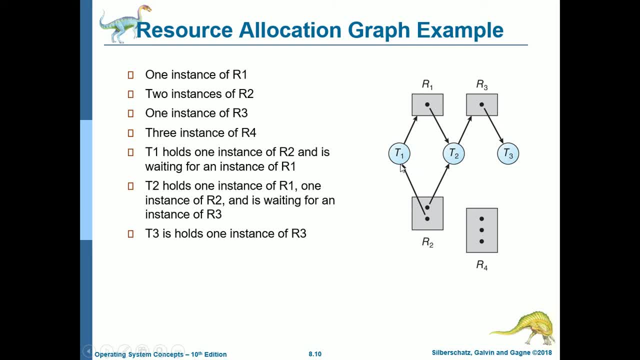 is assigned to T1, meaning thread 1 holds an instance of R2.. And we have also an arrow going from T1 to R1, meaning that T1 requests for another resource of R1, or rather waiting for an instance of R1. And then T2.. So for T2.. So 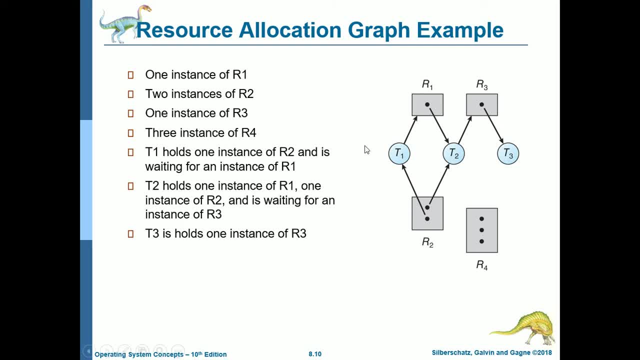 it holds one instance of R1. As you can see here for the assignment edge of R1 going to T2. And then T2.. So it holds one instance of R1. And then T2.. So it holds one instance of R1. And then. 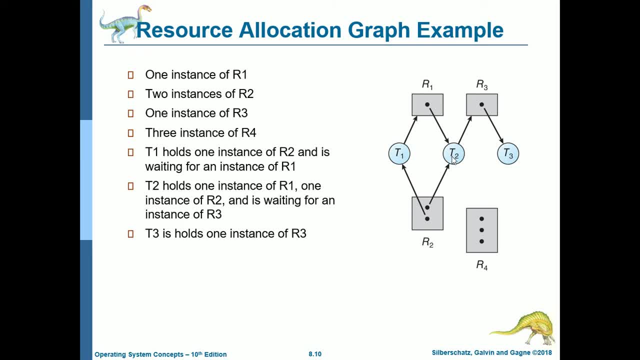 one instance of R2.. So it also has acquired the resource resource number 2. So it is assigned also to T2. And it also waits for the instance of R3.. And then T3 holds one instance of R3. 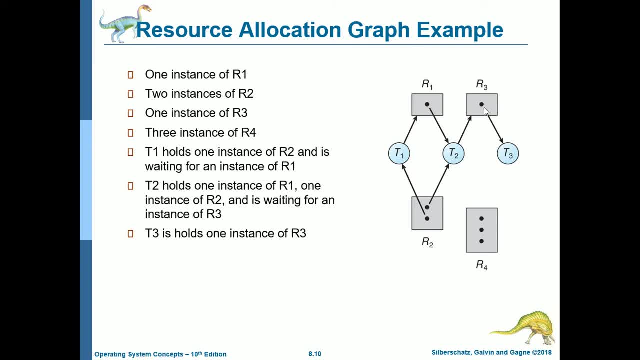 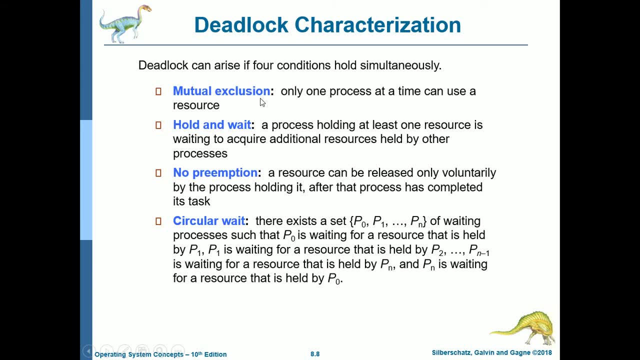 Okay for this resource allocation graph. So let's use the four conditions. that is stated again. So let's go back. We have the mutual exclusion, hold and wait. no preemption and circular wait. Okay for mutual exclusion. So it is said here: 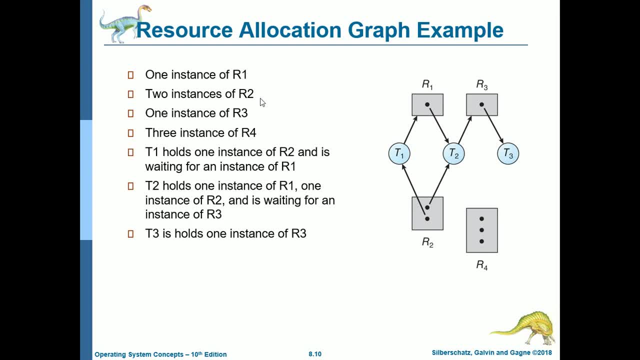 only one process at a time can use a resource. So of course, one instance of resource assigned to a thread or a process And then hold and wait. So is there at least one process or thread that is holding a particular resource and then waiting for another resource, that is 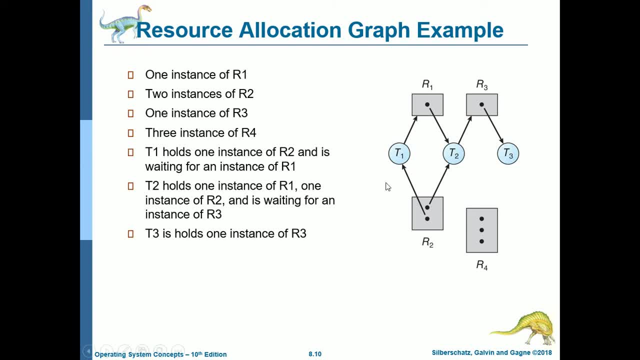 held by another process. So we have that instances for T1.. It already has R2, but it's waiting for R1, which is held by T2. And T2 already has R1 and R2 as its resource And it's. 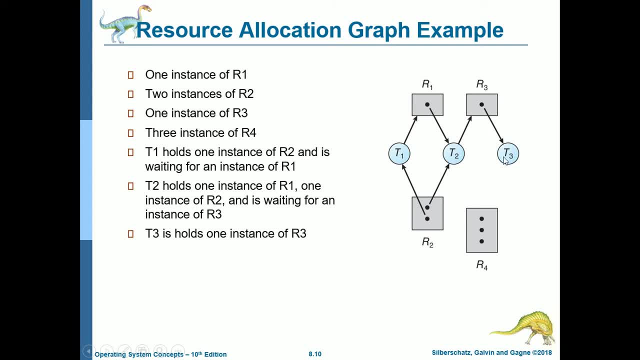 waiting, for instance, of R3, which is held by T3.. Okay, next is we have no preemption. So it is said that resources can only be released if a particular process or thread has finished its execution. So of course they haven't finished the execution. So 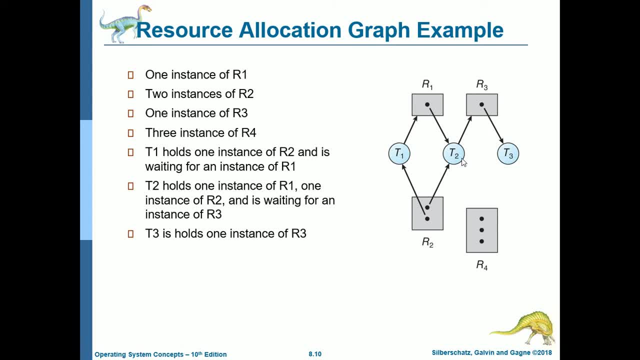 of course, they will not release these resources. And then the last one is circular wait. As we can see, it should be that T1 is waiting for a resource that is held by T2.. So we have this instance, that is, R3.. 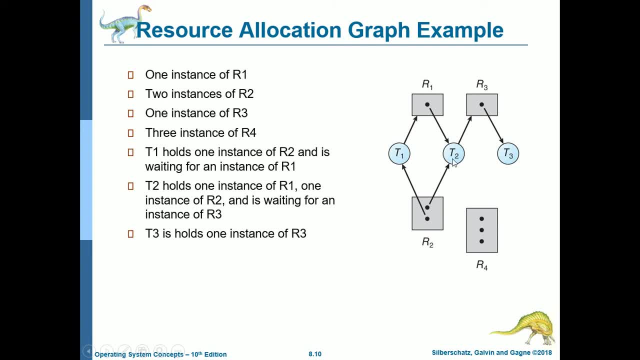 T1. And then is T2 waiting for a resource that is held by T3? So actually we have. we can see that in here. So is T3 waiting for a resource that is held by T1? Actually? 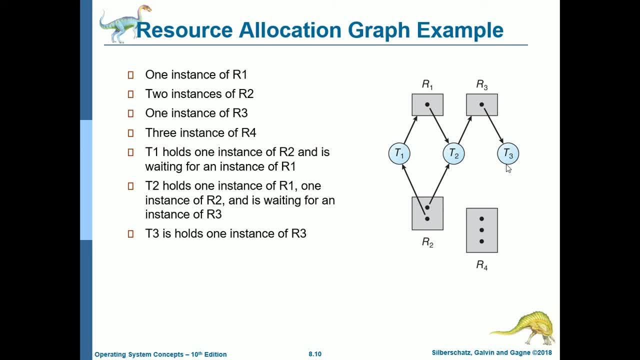 for T3, it does not. So can we conclude that is there a deadlock? Is the setup of the threads here has a deadlock? Actually, there is no deadlock because it does not have a circular wait, Because it should have been. if T3 has an arrow going to R2, then there is a possibility. 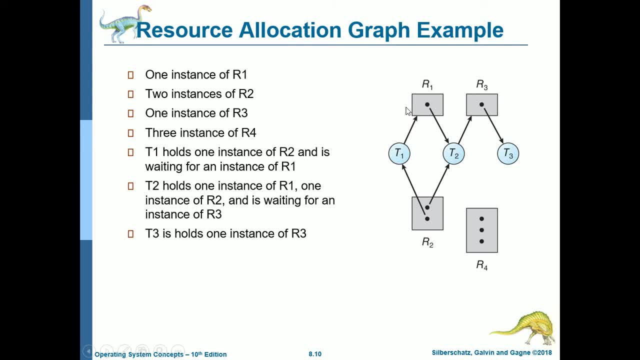 of deadlock Because it really has a possibility of deadlock, Because T3's resources is waiting for the resource that is held by T1. So for this particular process it should have been a deadlock. So for this particular example there is no deadlock because the circular 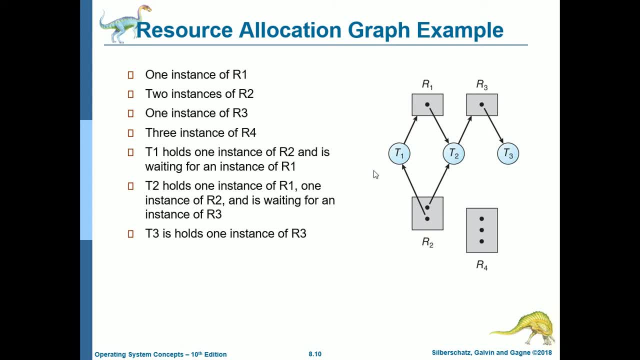 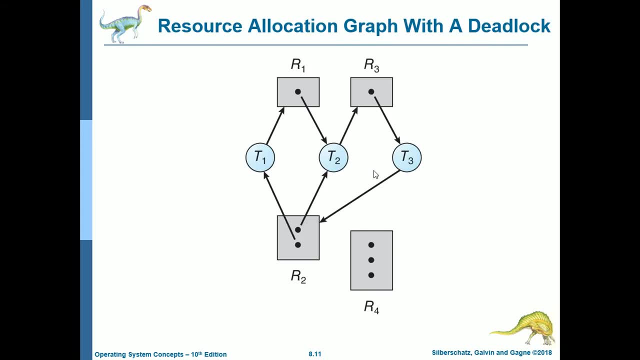 wait, here is not is false, Because it means that all processes, or rather threads, Okay. So we have a resource allocation graph with a deadlock. So this is a modification of the previous resource allocation graph. So, as I already said, this will have a deadlock. 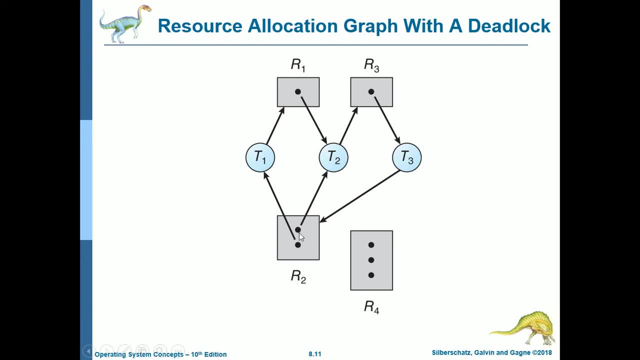 because T3 needs a resource that is held by T1. So it is already. it already has a circular wait, So let's check. So again, mutual exclusion: So a process or thread should hold process one at a time. So we have that, And then 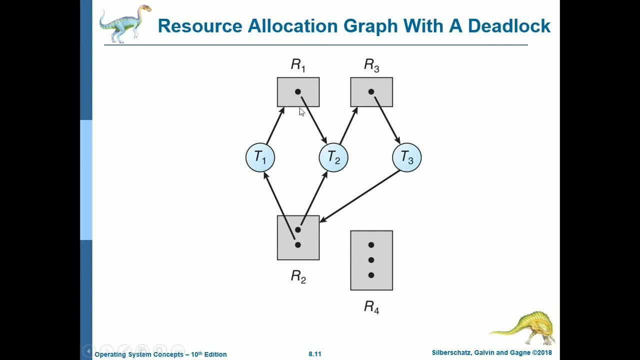 and then they cannot. for example, if this one instance already assigned to R2, they cannot share. So that is the meaning of mutual exclusion. Then we also have hold and wait. T1, T2, and T3 have these conditions that they already have a process waiting for. 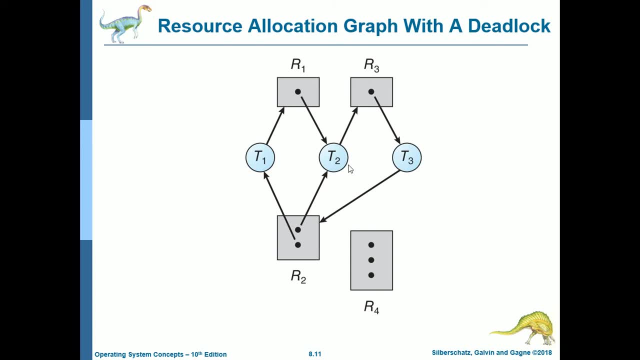 the process that is held by rather waiting for a resource that is held by the other process, And then no preemption. There is no release again of resources unless the threads or processes has finished its execution And circular wait. So T1 needs a resource that. 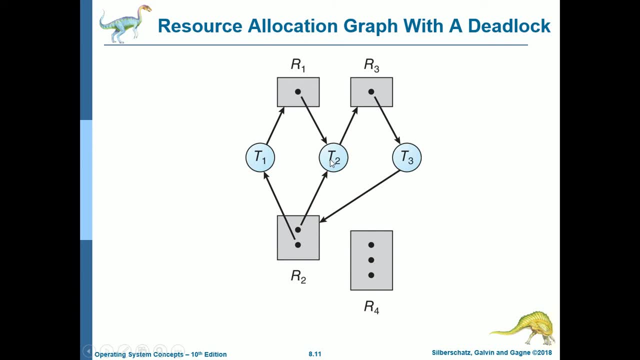 is held by T2. And then T2 needs a resource that is held by T3. Then T3 needs a resource that is held by T1. So it's already a circular wait. So this definitely has a deadlock. 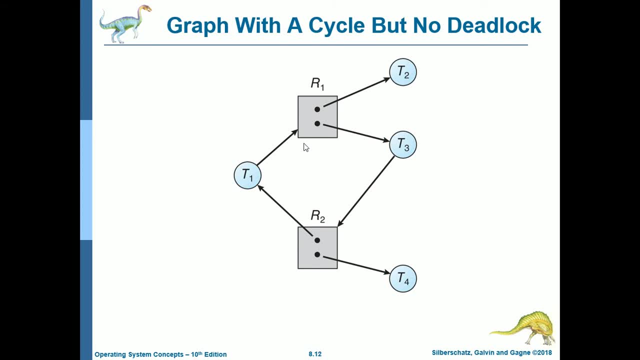 Okay. Next is we have graph with a cycle but no deadlock, So okay. So let's check again the four characteristics of a deadlock: mutual exclusion. So each of the resources is assigned to only one thread. So that is why. So R1 is assigned. 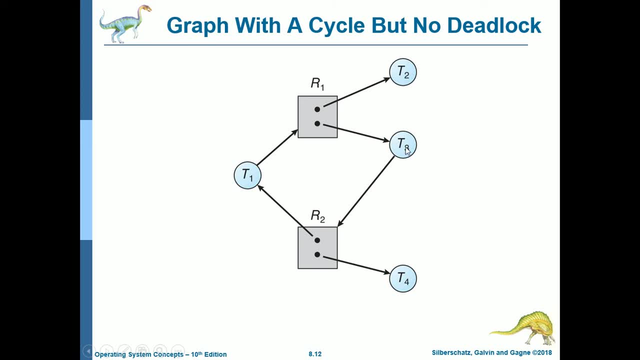 to T2.. Another instance of R1 is assigned to T3. And then R2 is assigned to T1. And another instance of R2 is assigned to T4. So that is already mutual exclusion. Then next is we have hold and wait. So does T1- already has resources, Of course R2.. 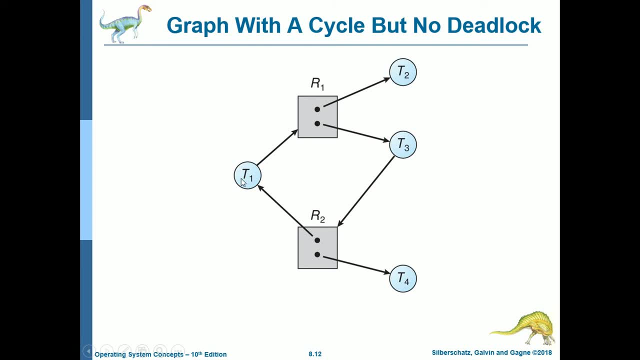 And then T1 is waiting for the resources. that is held by other threads or processes. So R1 is needed by T1. It is held by T2 and T3. And also T3 already has a process rather. 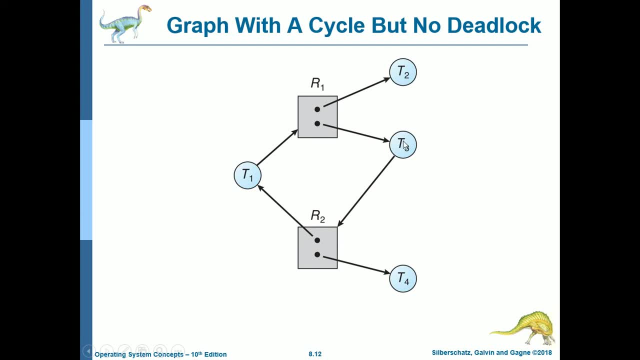 resource of R1. And it needs additional resources: R2, which is held by T1 and then T4. So it also has a hold and wait. Next is Nope, please preemption. so again, for no preemption, that the processes, uh and threads will not release its. 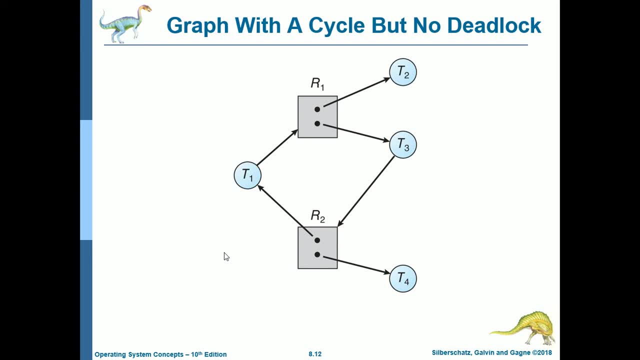 resources allocated as long as they are not yet finished with their uh execution. so that is that it. that is um, no preemption. and then we have the last circular wait. so circular wait, okay, does t sub one needed uh, a resource that is held by t sub two? yes, but this does t sub two. 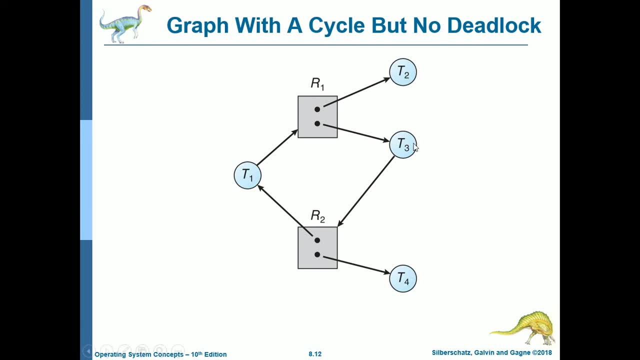 um wants a resource that is held by t sub three actually? uh, it's not true, because it only needs one resource from r sub one. does t sub three holds a resource held by t sub four? yes, but t sub four does. does need a resource that is held by t sub 1? actually, no. so, though, this example has a cycle, as you can see. 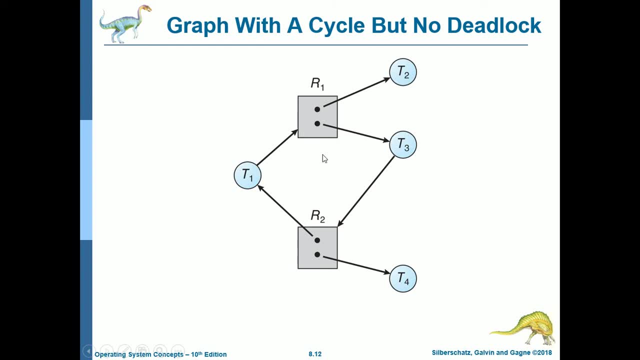 here for the t sub 1, t sub 3, but it does not have a deadlock because it does not satisfy the requirement of deadlock characterization, which is circular weight. and this it has no also deadlock, since if t sub 2 and t sub 4 is finished its execution, then t sub 1 will acquire the resource. 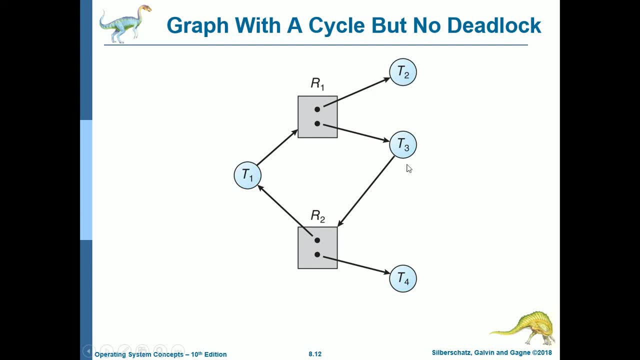 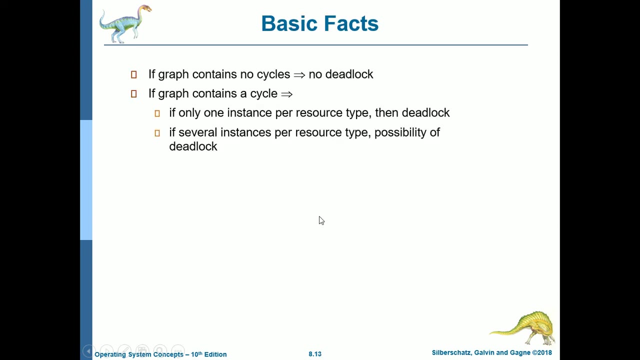 that is released by t sub 2 and the resource released by t sub 4 will be acquired by t sub 3, so there is no deadlock. so this example: there is no deadlock, even though there is a cycle. so basic, basic facts. so if graph contains no cycles, definitely there is no deadlock. so if 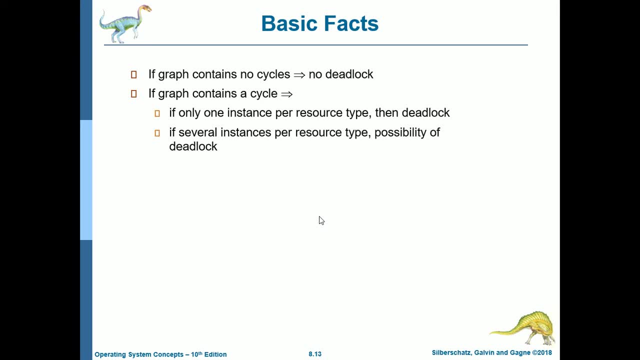 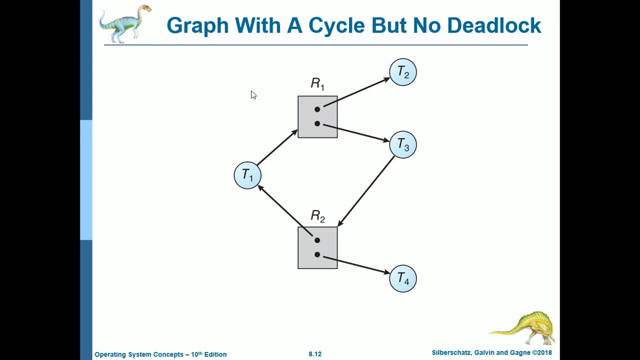 graph contains a cycle. so, as you can see though, in the in the example, there is a cycle, but there is no deadlock, because it does not satisfy the four deadlock conditions for dead for the deadlock. so, okay then, if, if a graph contains a cycle, if only one. 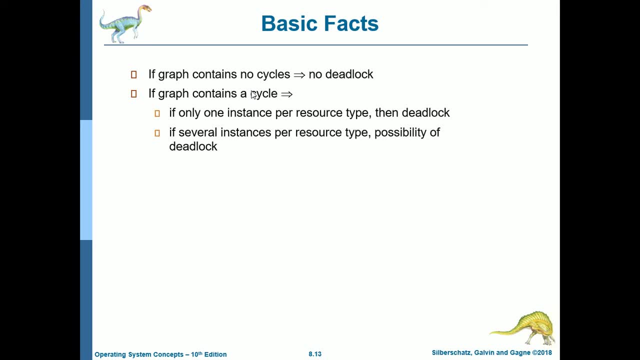 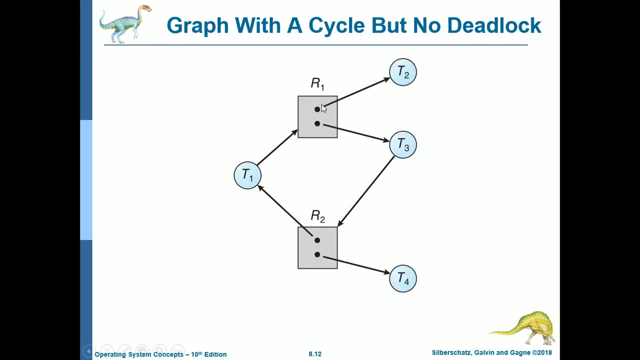 instance per resource type, then deadlock. so specifically, if the resource type is or has only one instance, then definitely there is a deadlock. so for this example, since the resource type is deadlock, it is also deadlocked. so if t sub 2 is already finished its execution, then they. 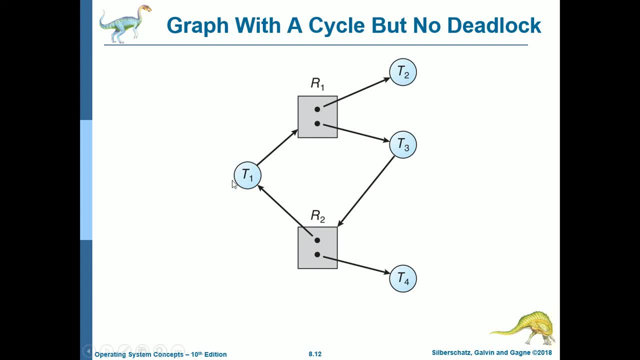 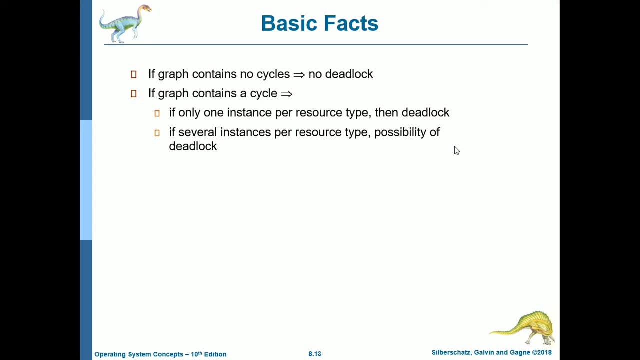 don't need to wait for the resource. it will be allocated to the processes that or threads that needed that particular resource. then if several instances per resource type, there is a possibility of deadlock possibility but not definitely there is already a deadlock because again in the example that that is illustrated here, that 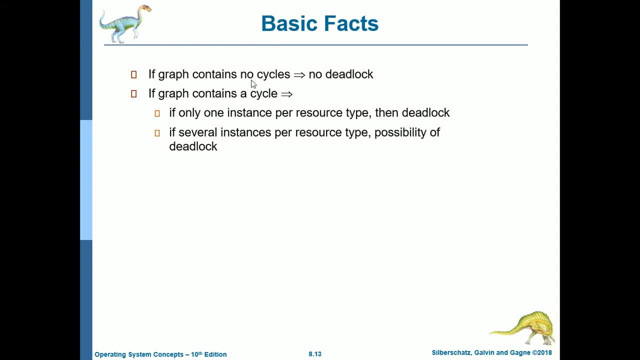 the resource type is deadlocked. so if t sub 2 is already finished its execution, then it will be allocated to the processes that or threads that needed that particular resource. so if t sub 2 is already finished its execution, then it will be allocated to the processes that or threads that. 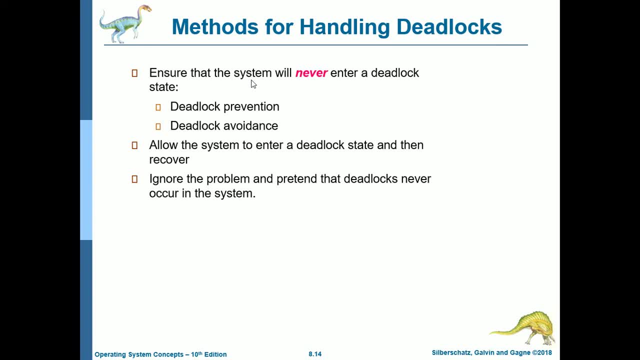 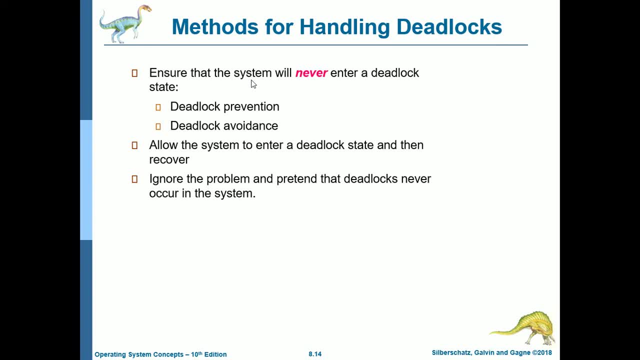 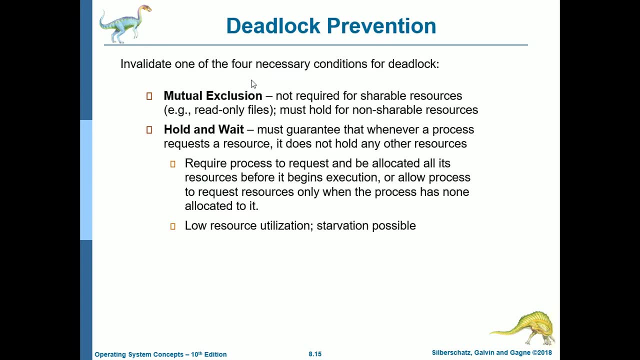 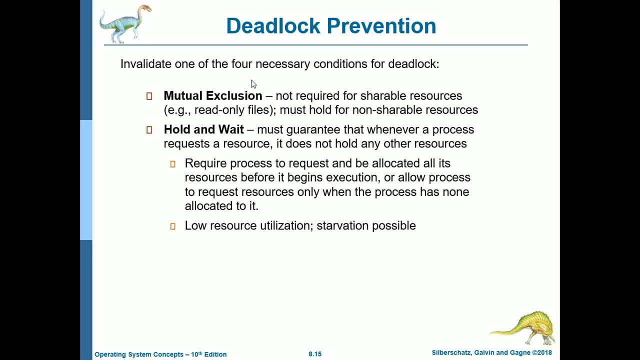 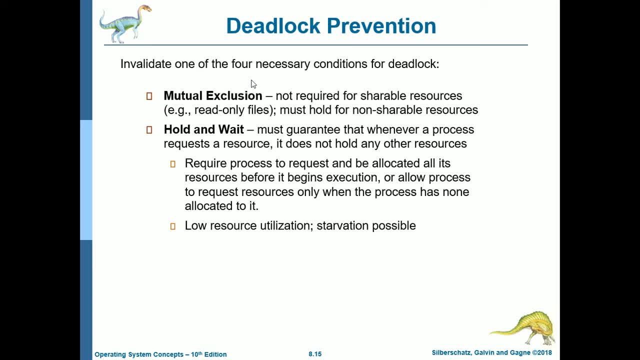 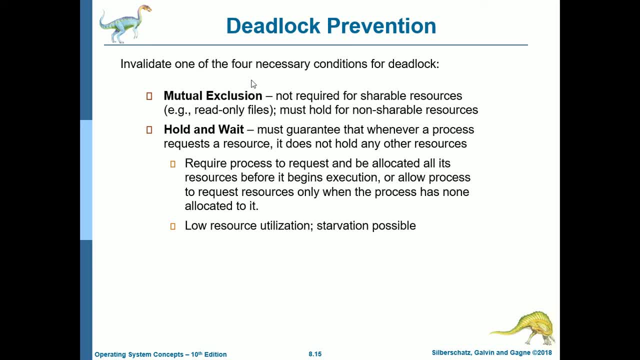 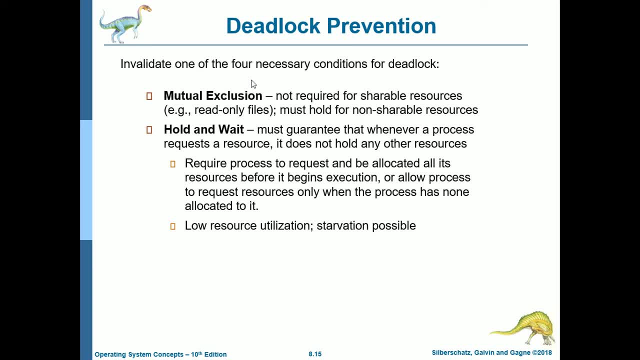 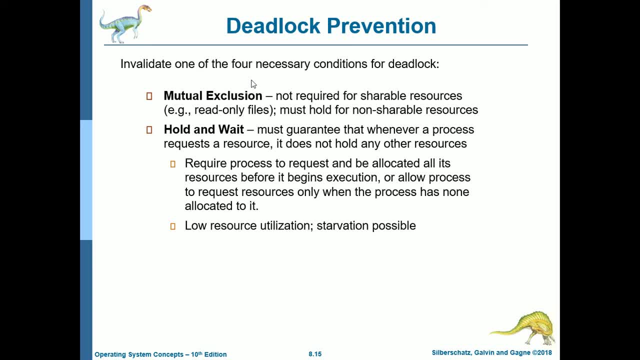 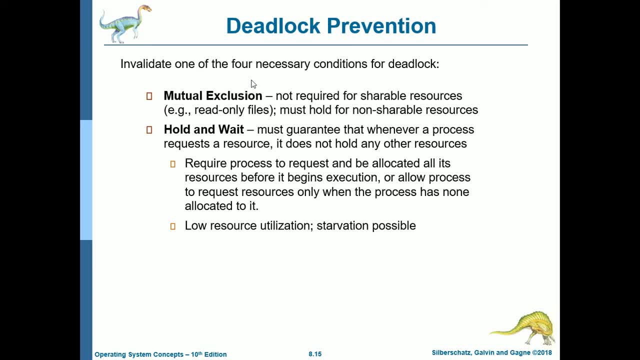 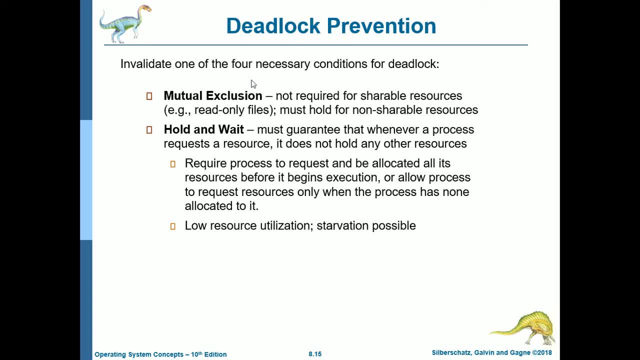 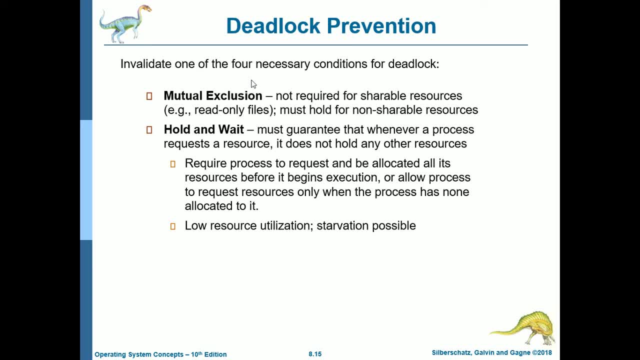 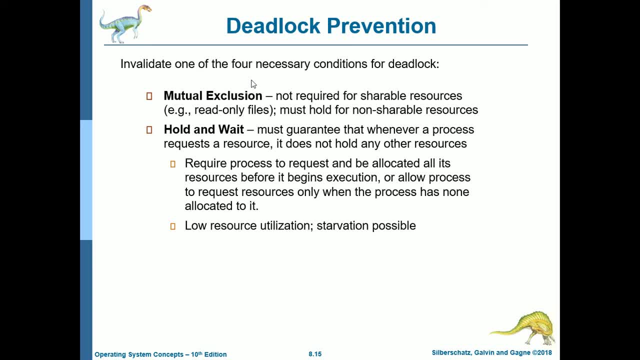 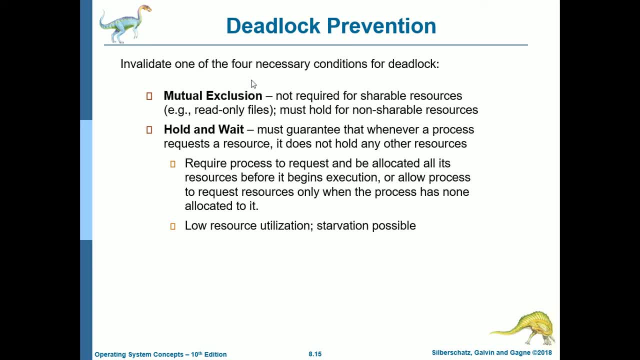 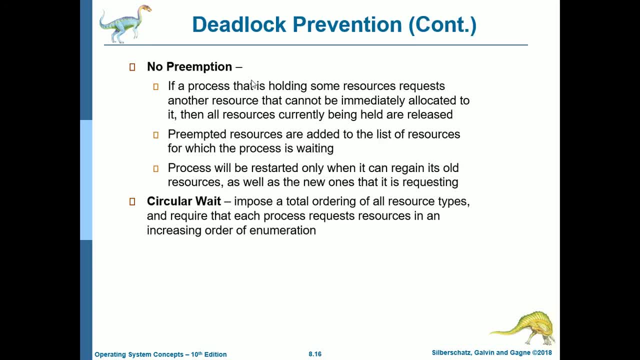 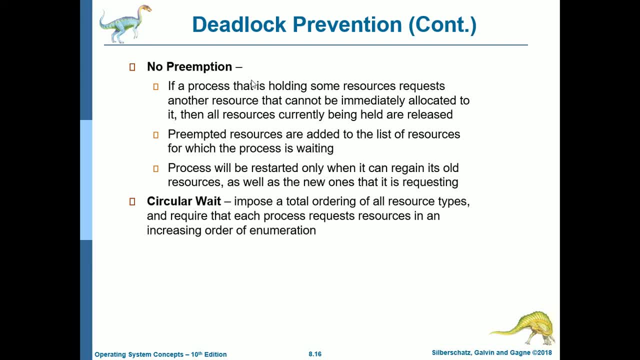 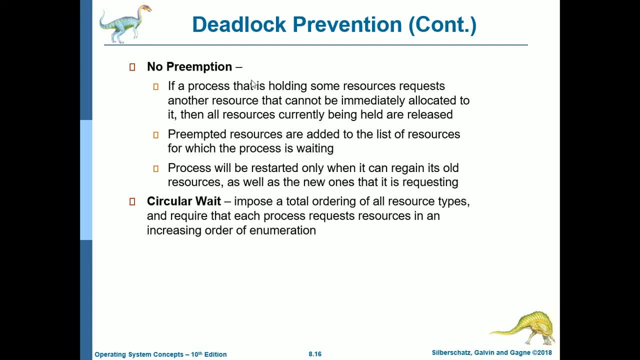 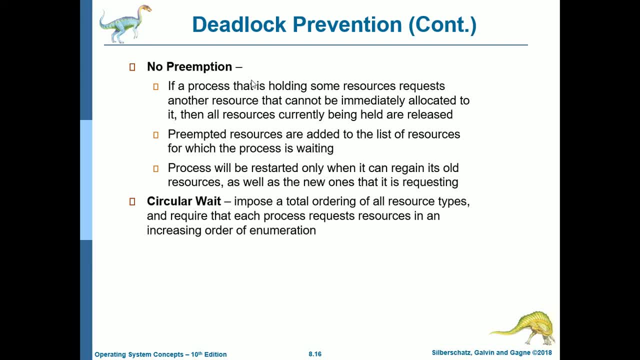 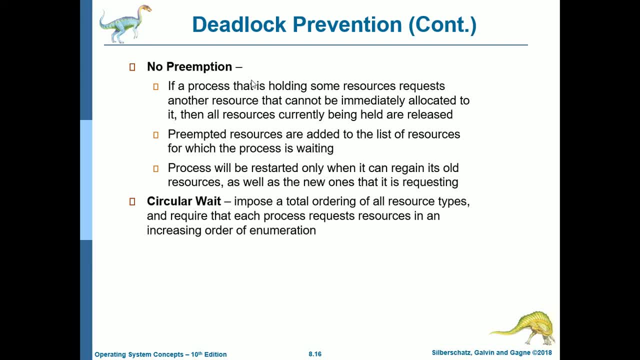 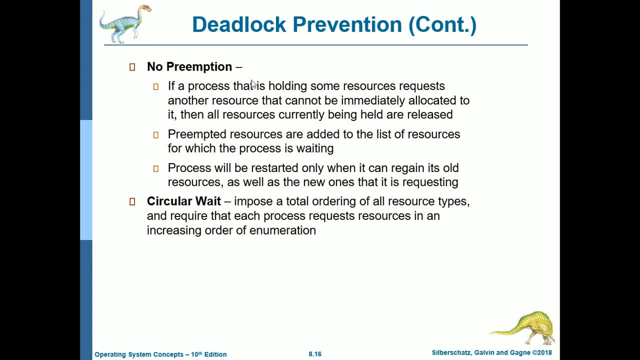 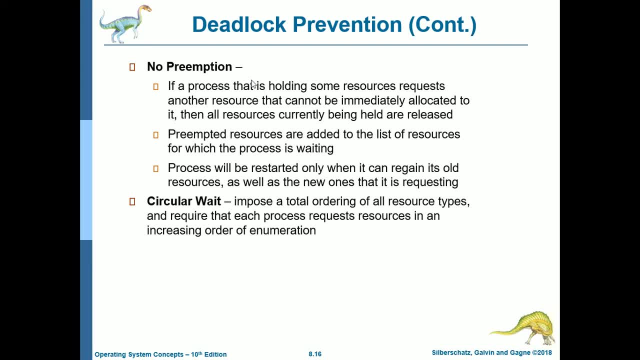 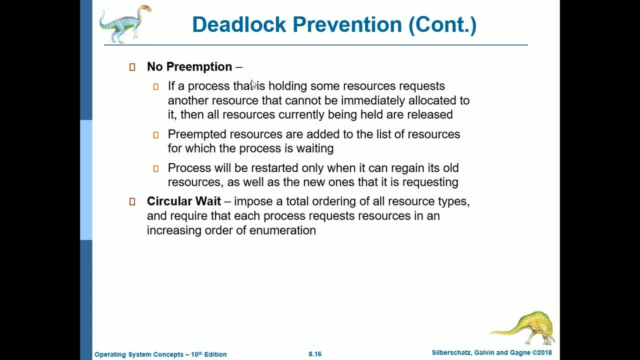 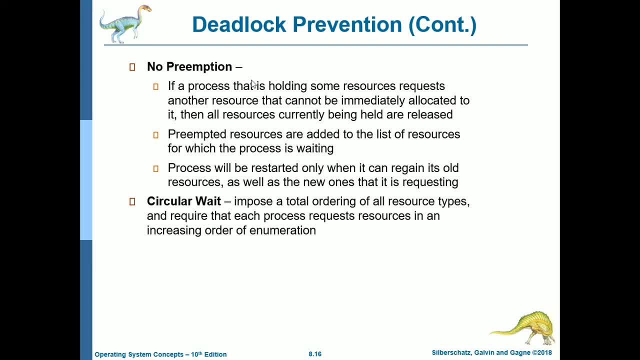 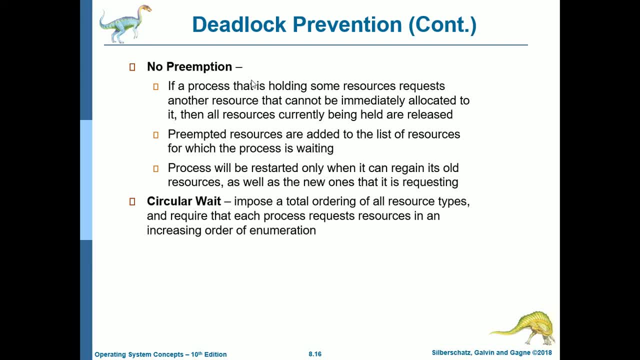 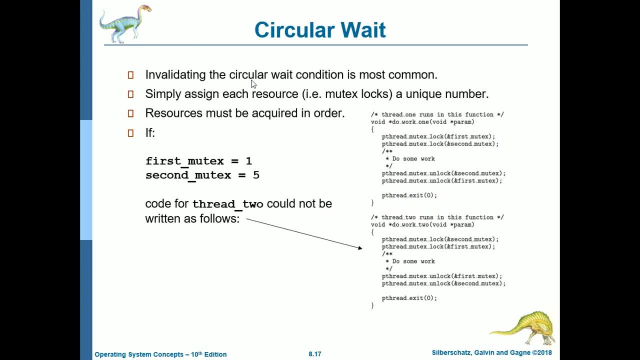 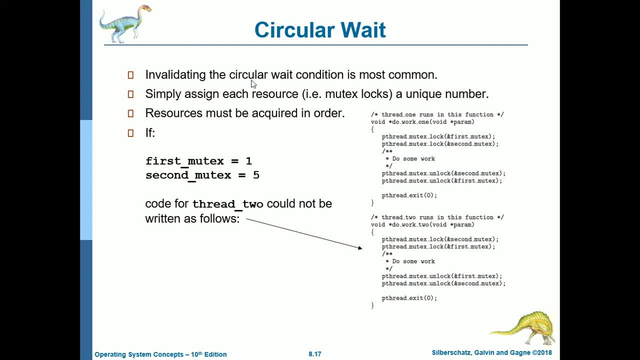 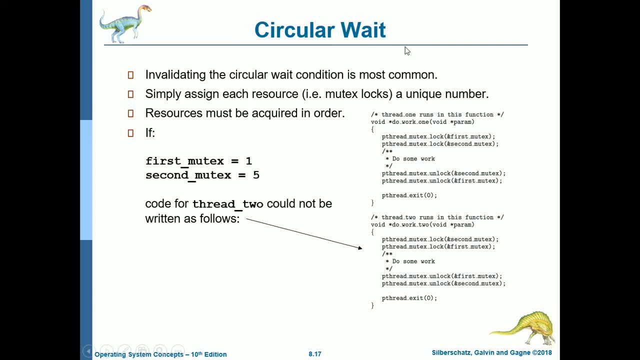 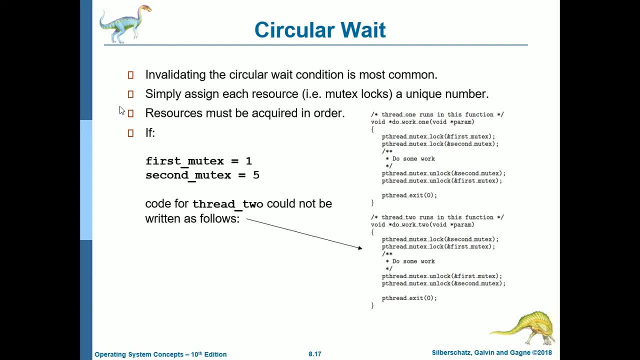 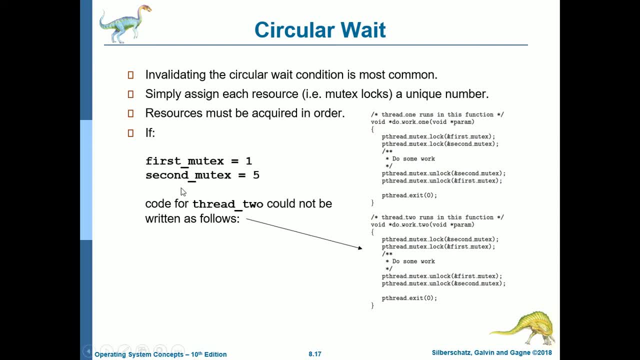 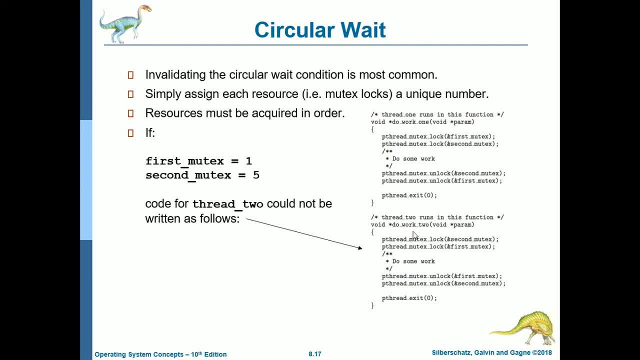 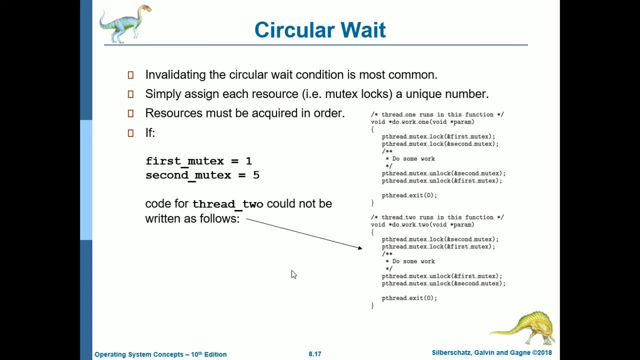 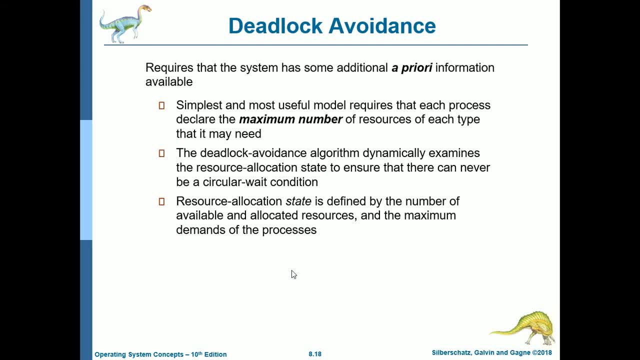 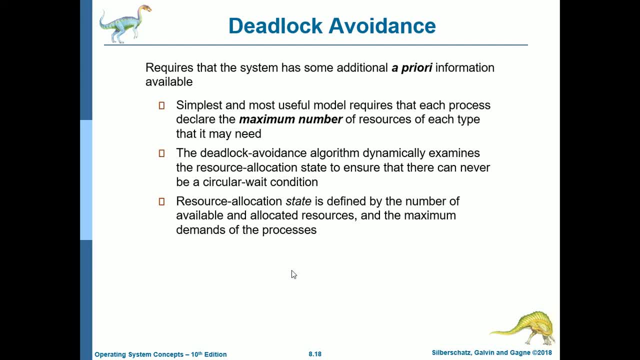 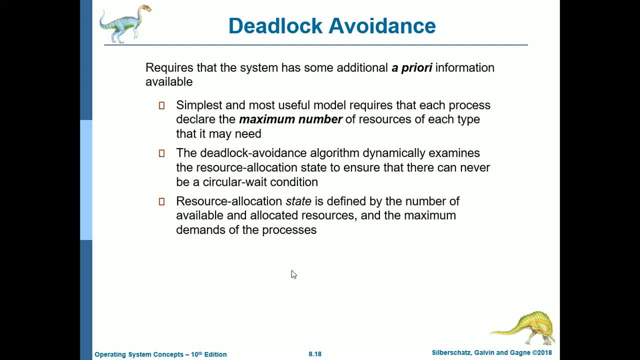 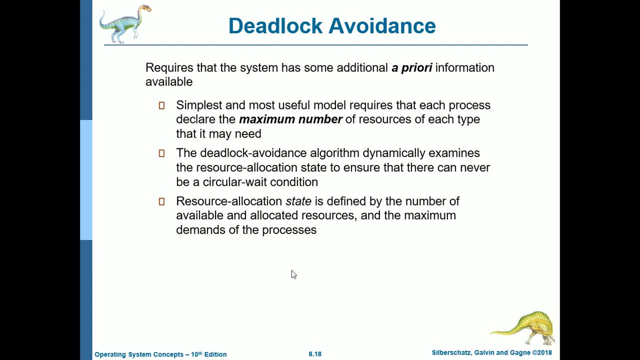 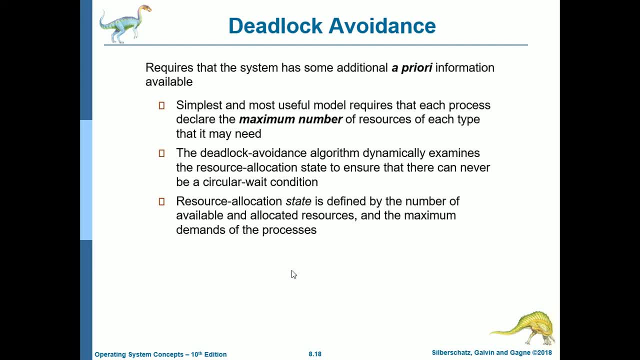 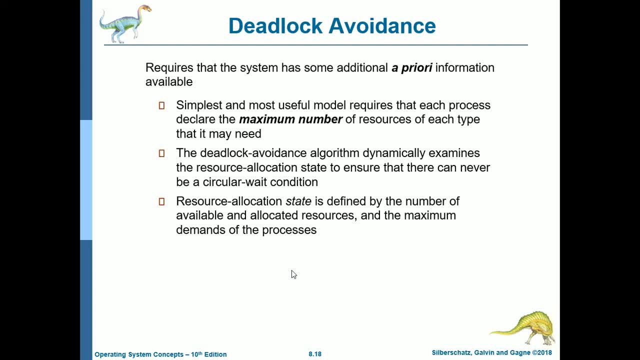 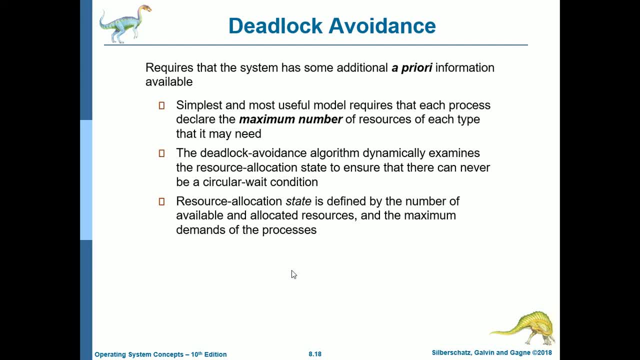 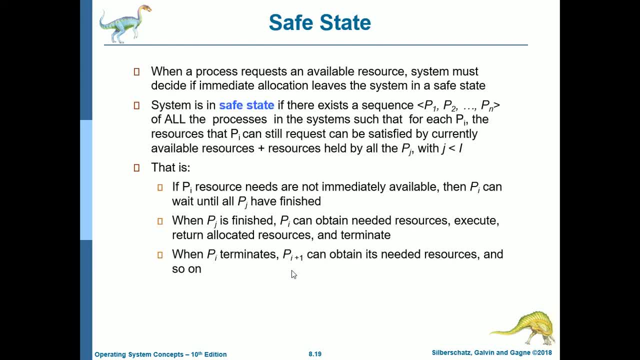 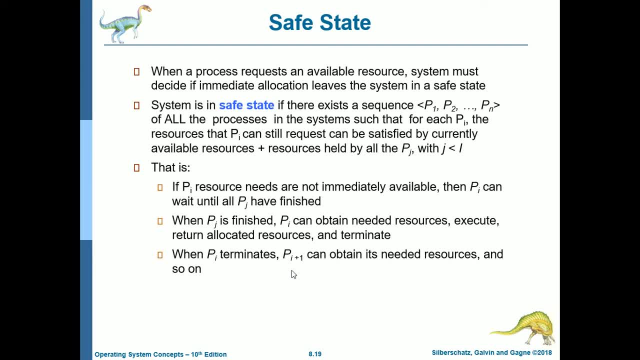 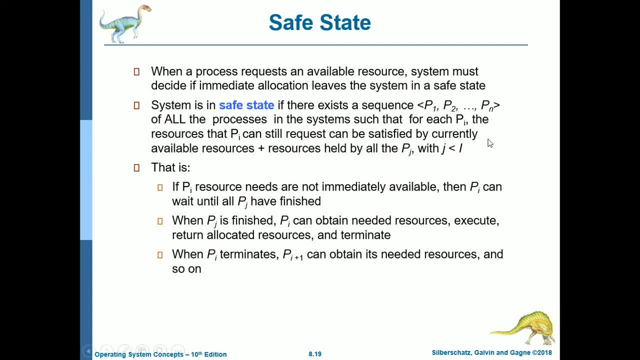 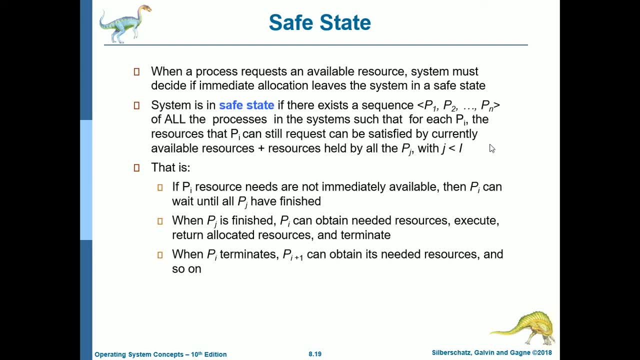 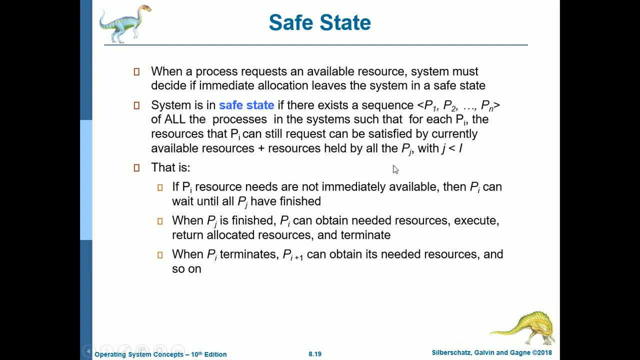 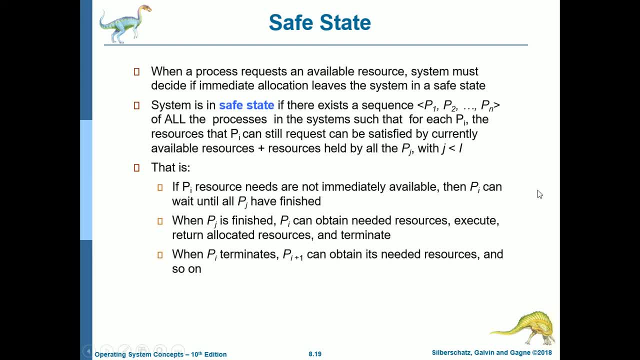 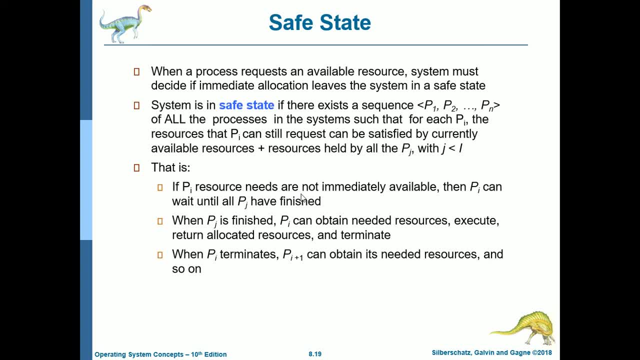 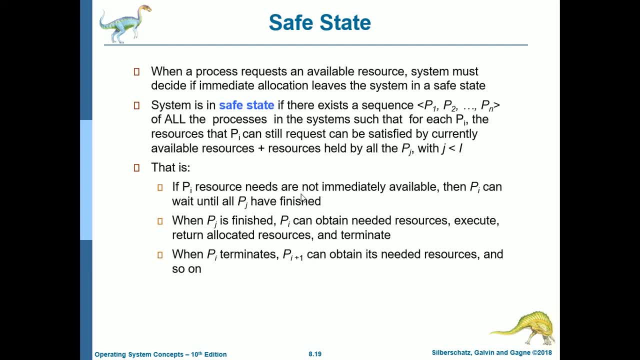 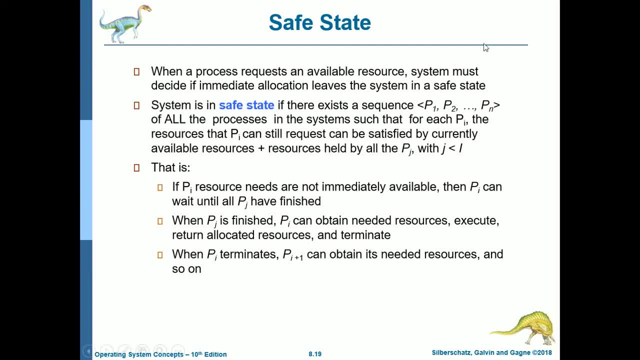 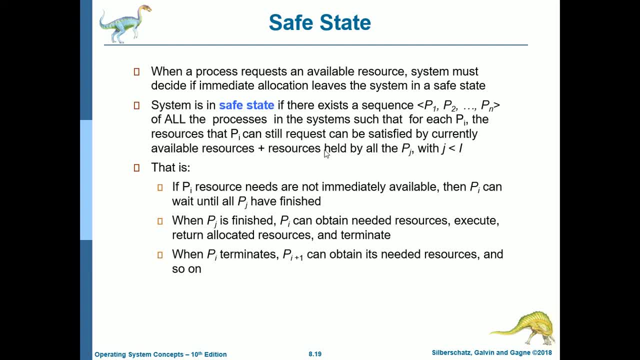 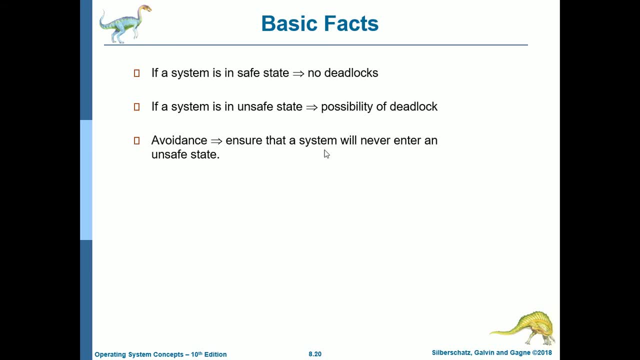 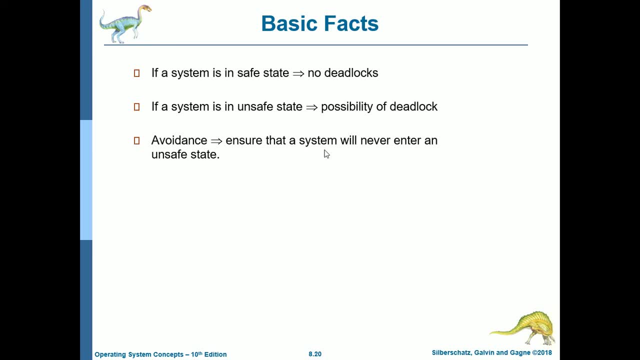 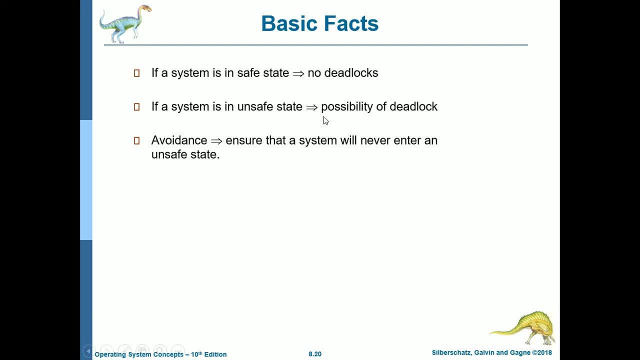 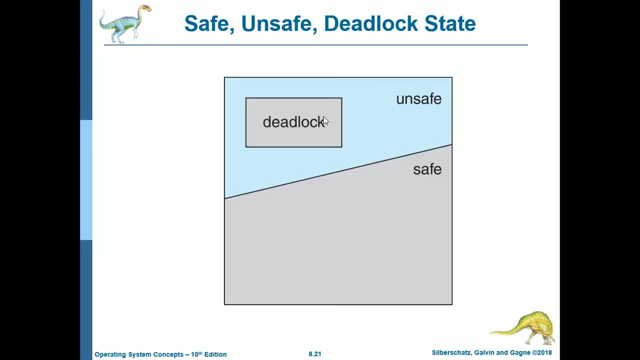 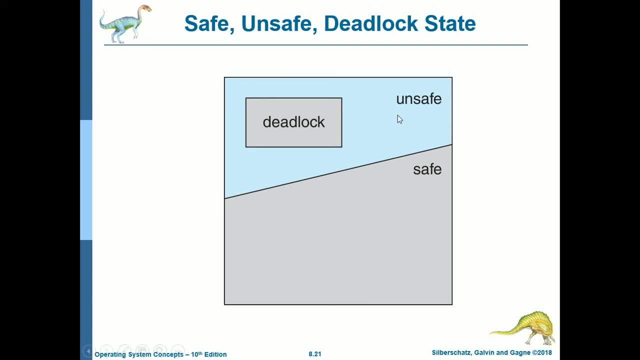 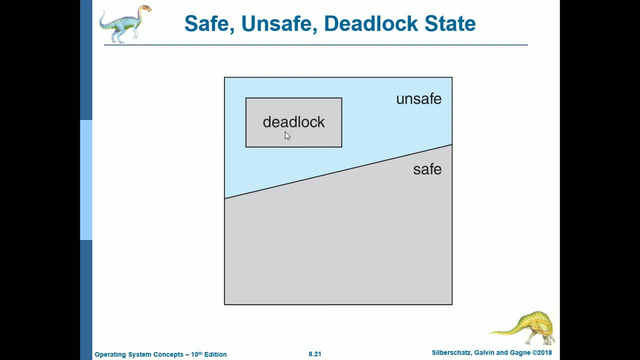 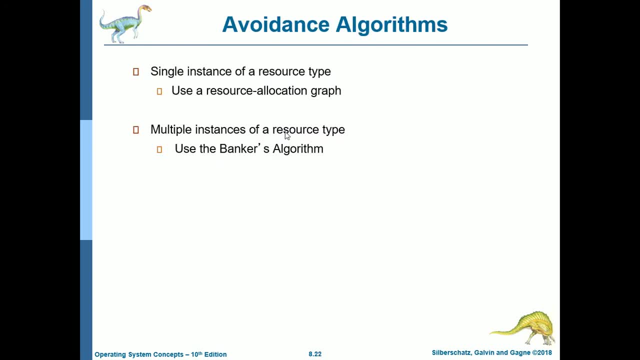 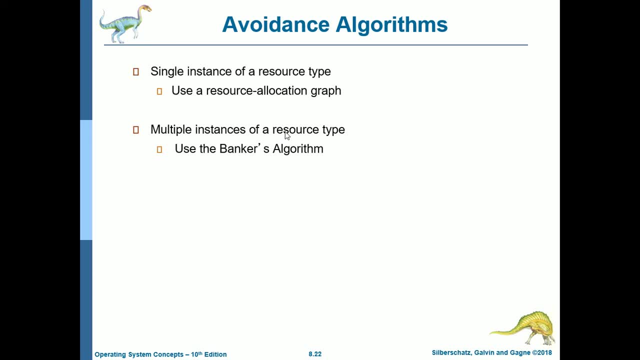 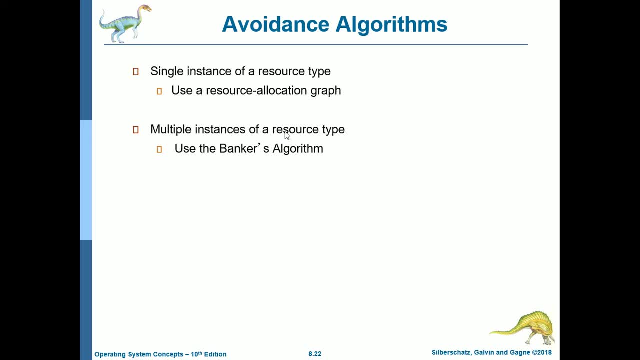 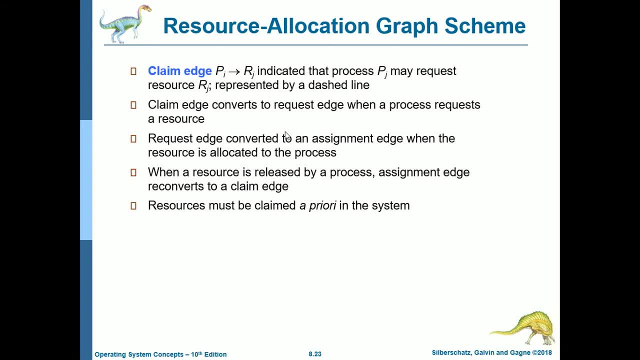 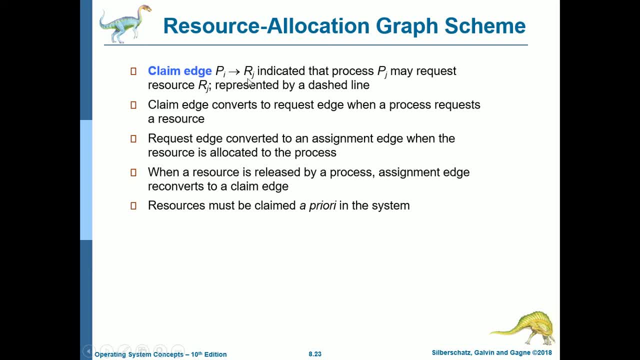 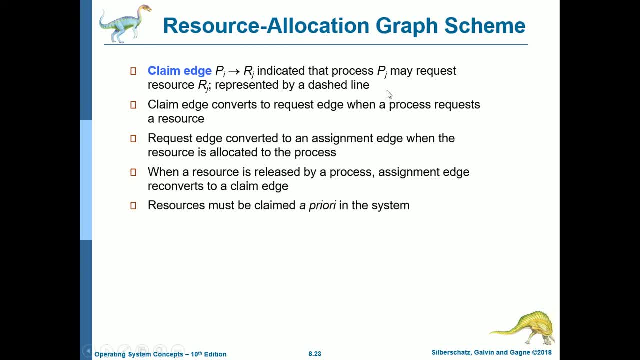 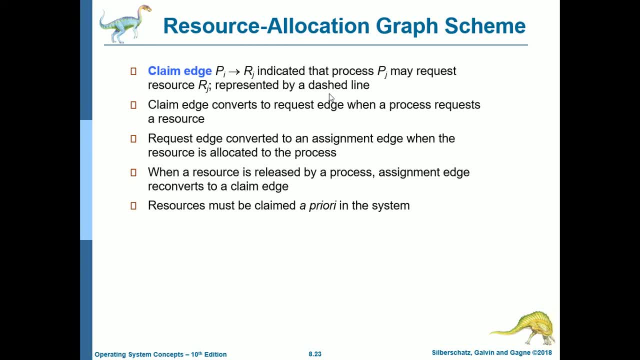 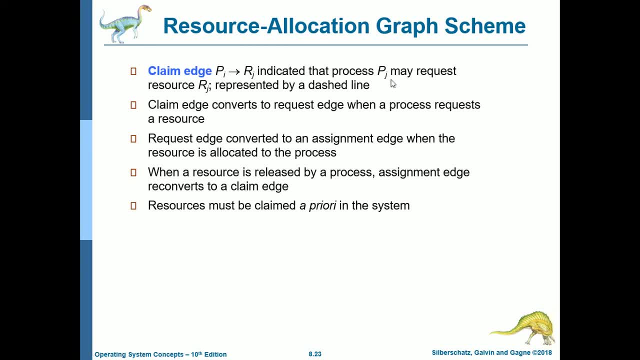 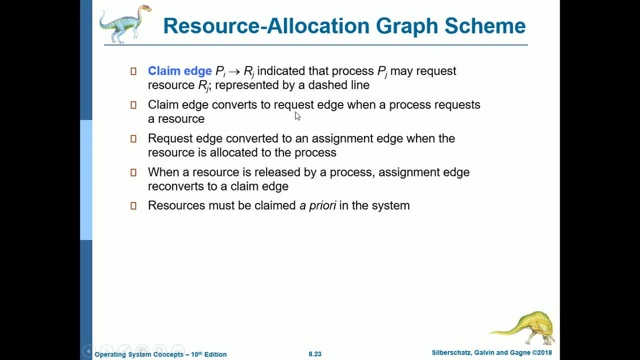 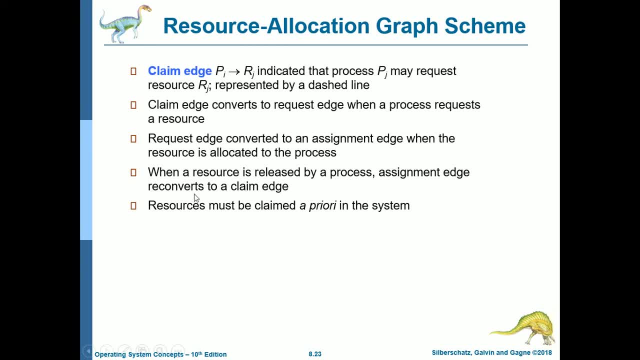 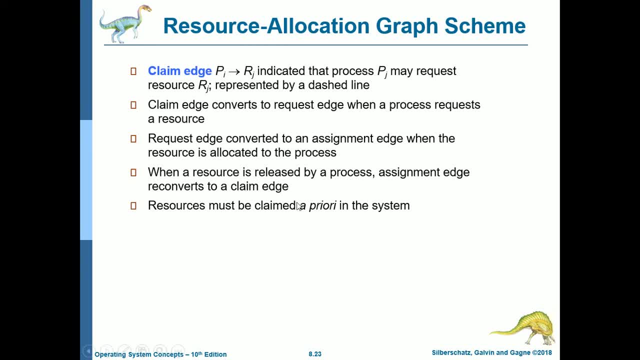 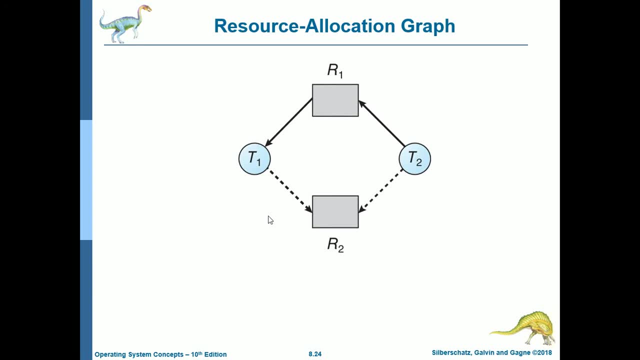 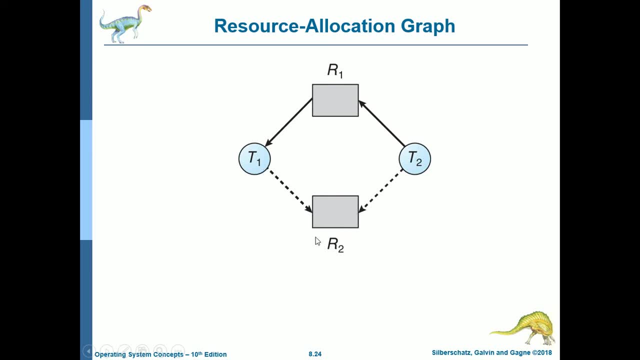 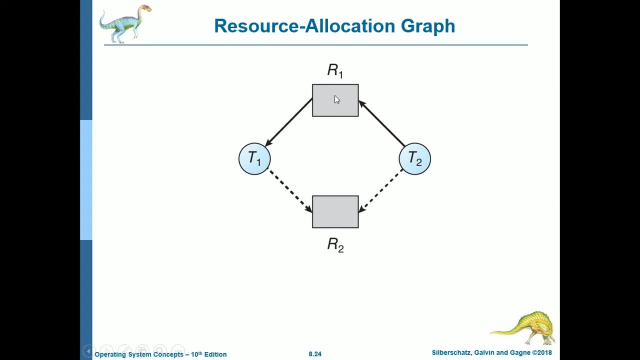 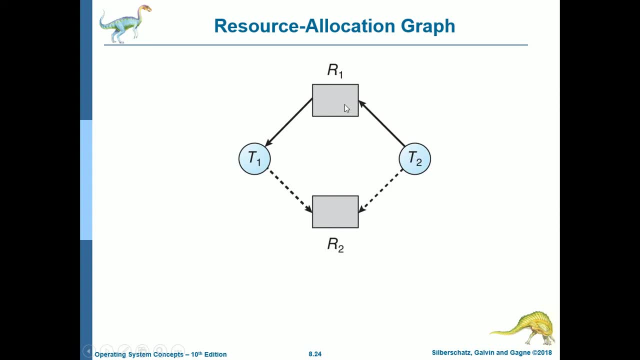 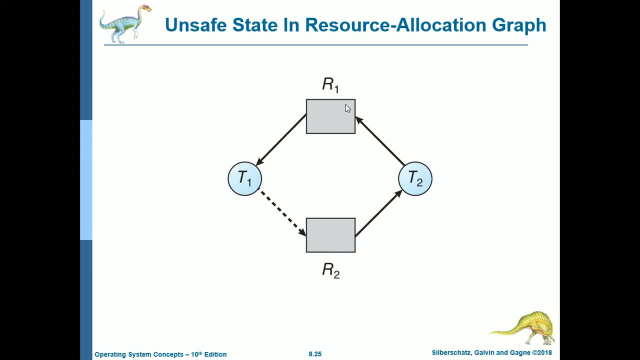 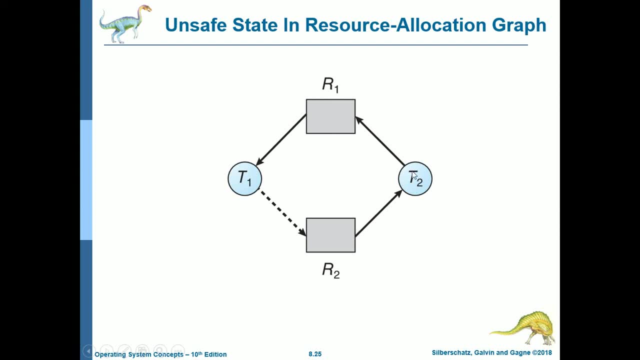 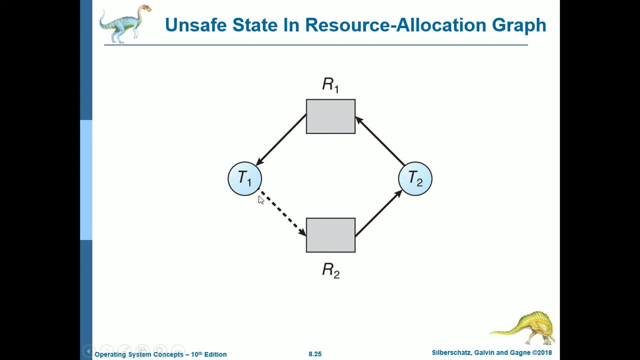 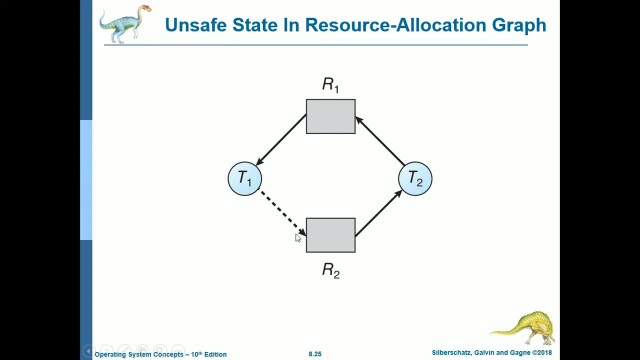 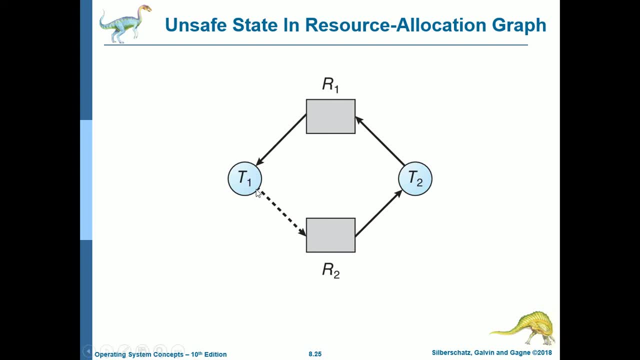 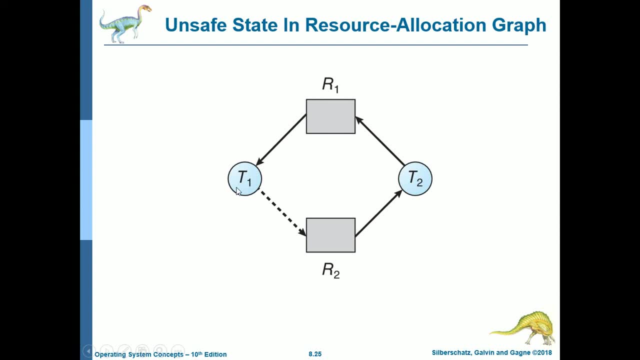 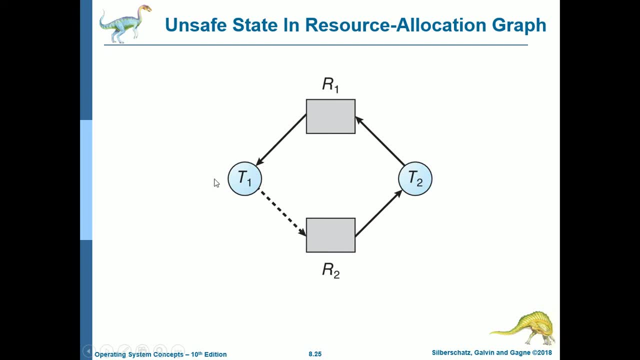 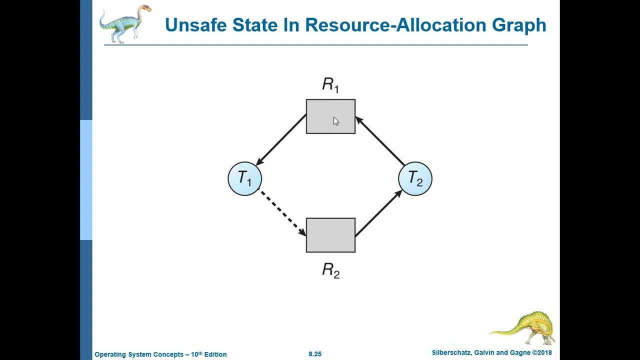 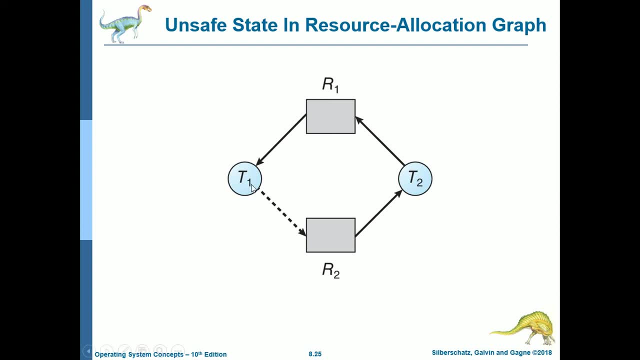 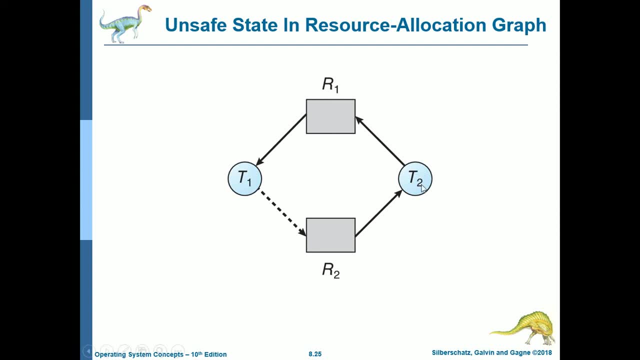 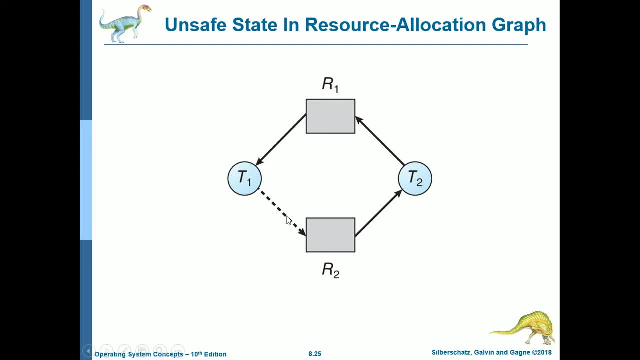 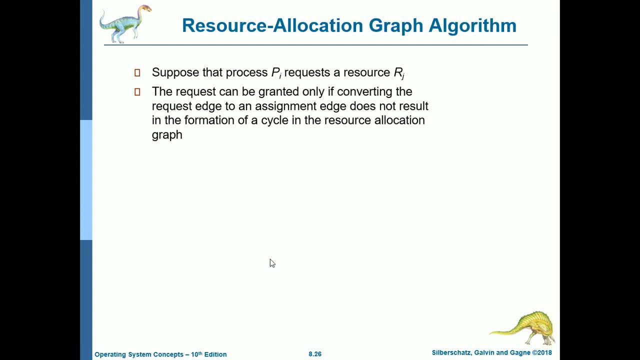 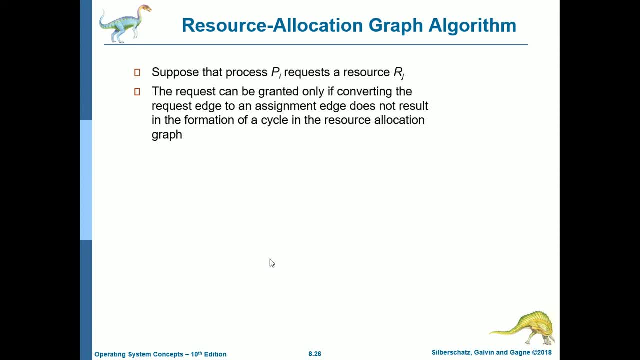 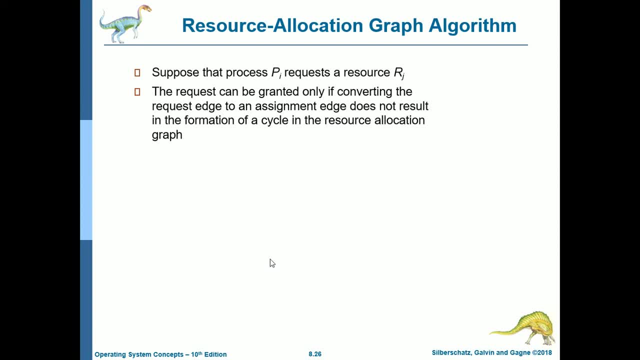 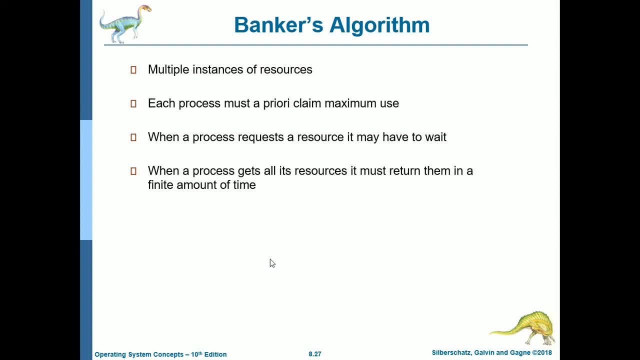 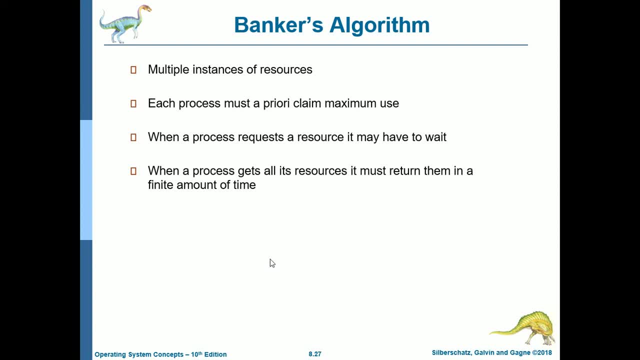 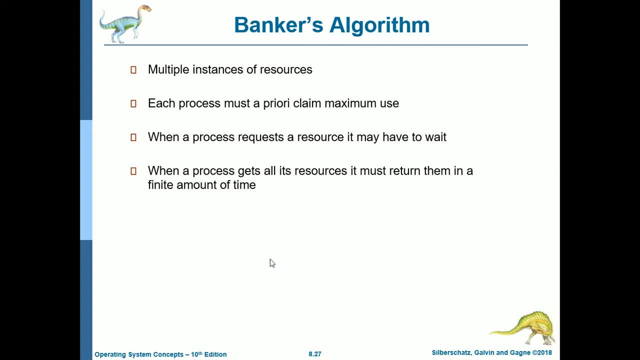 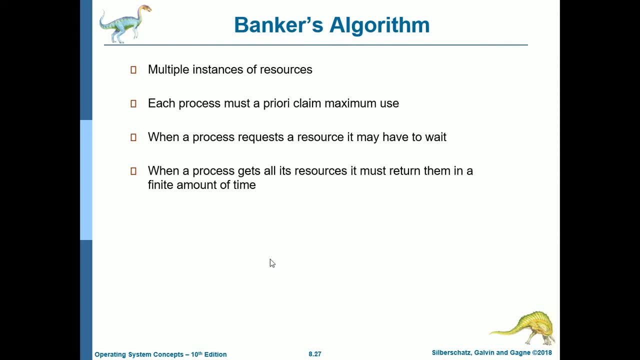 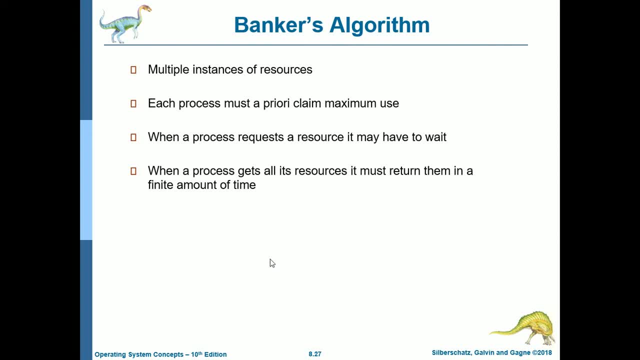 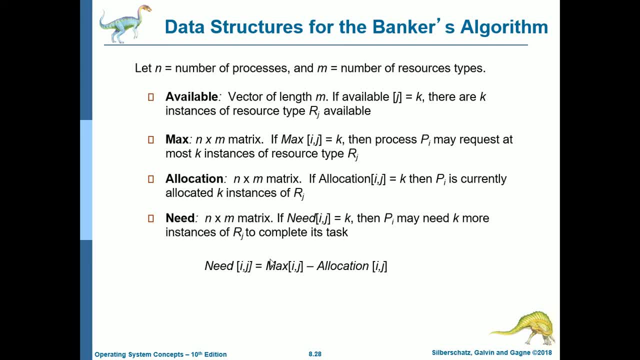 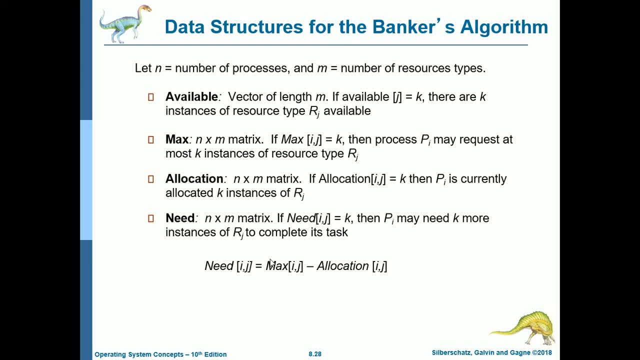 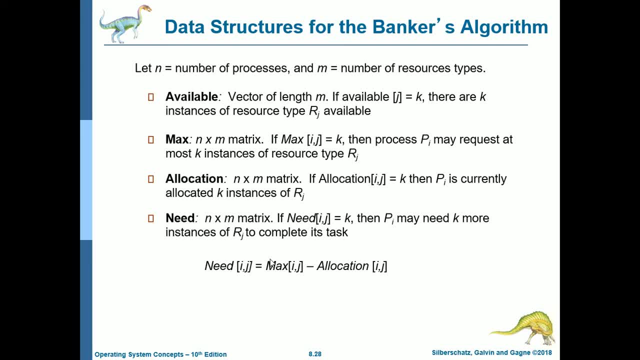 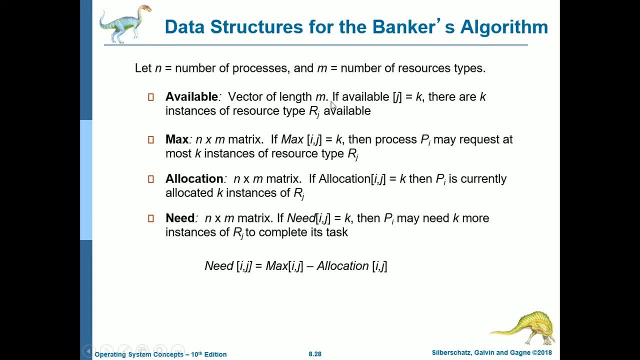 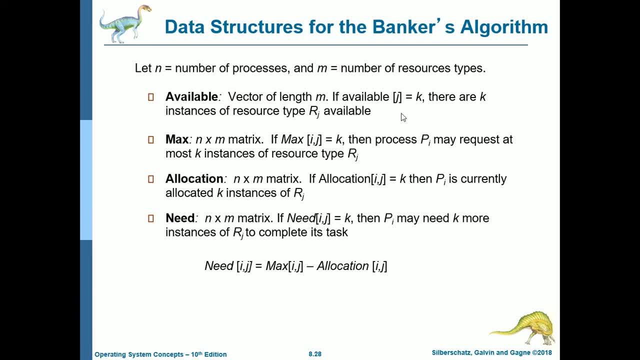 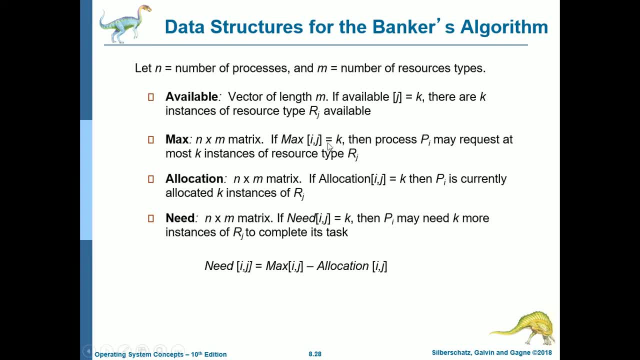 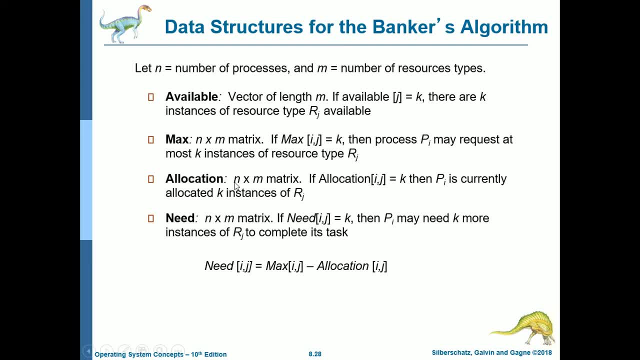 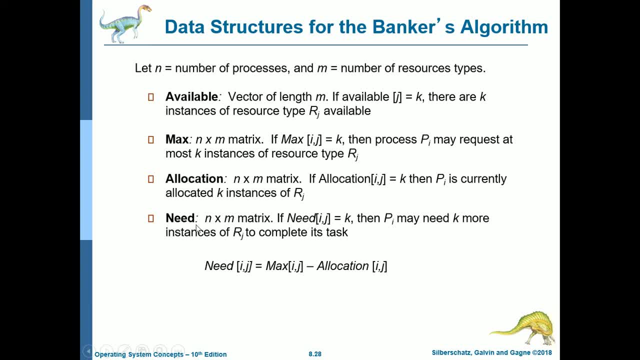 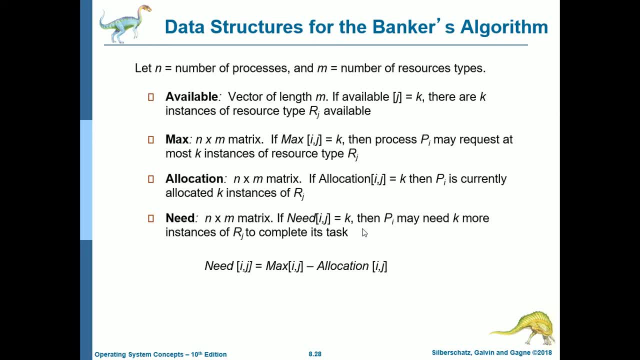 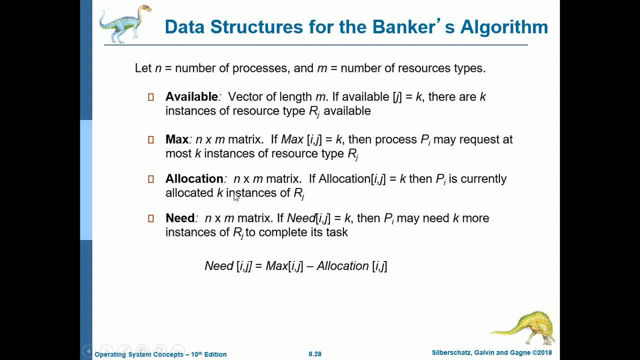 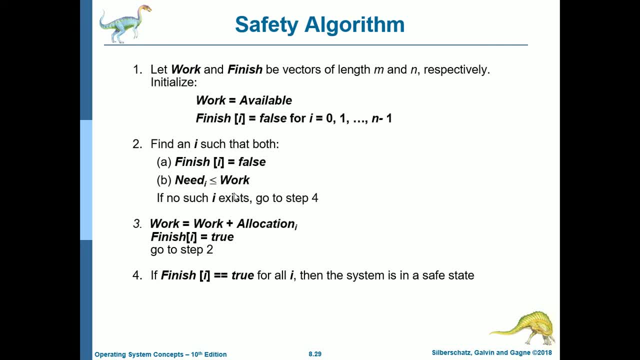 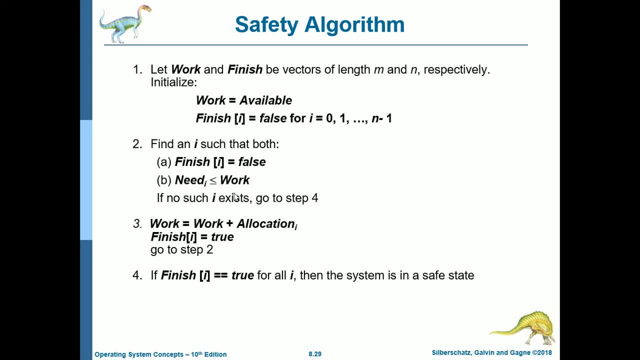 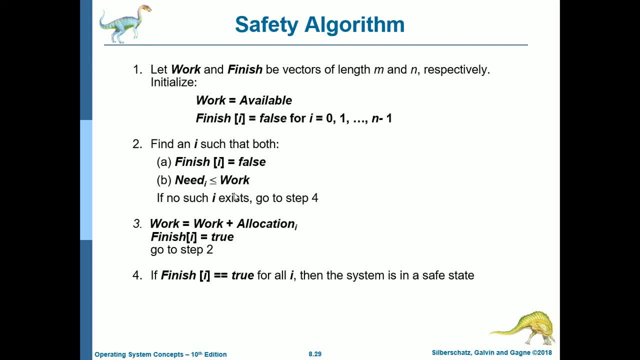 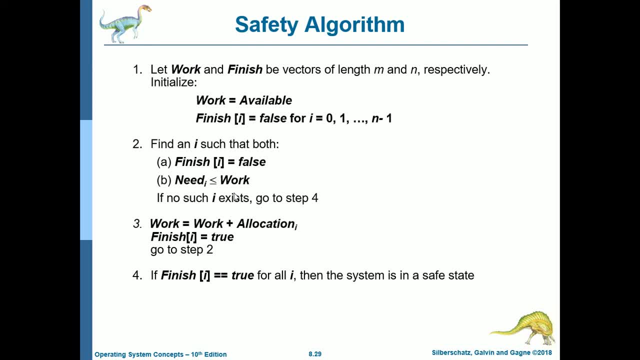 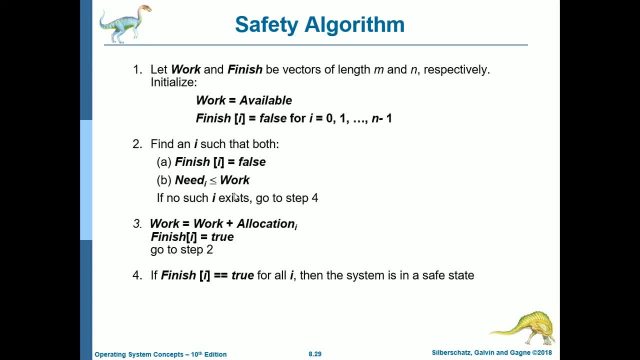 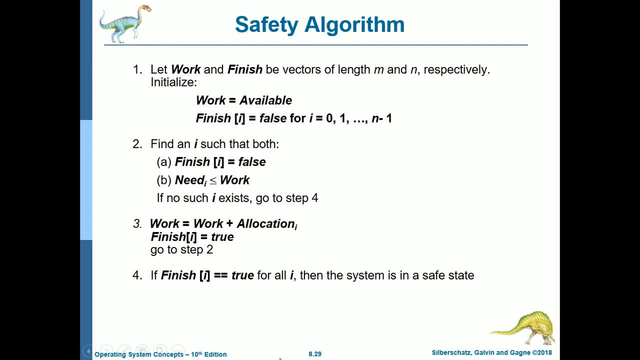 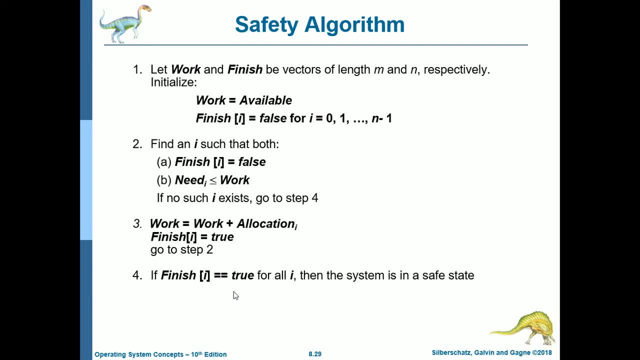 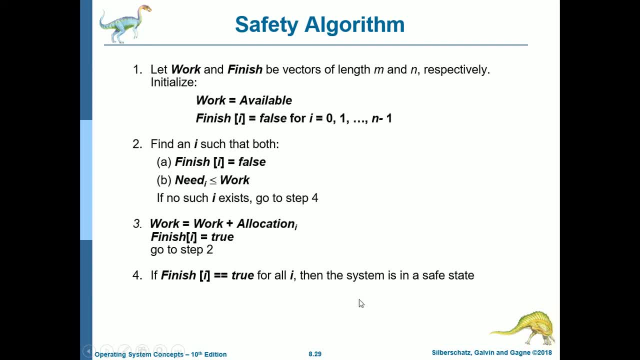 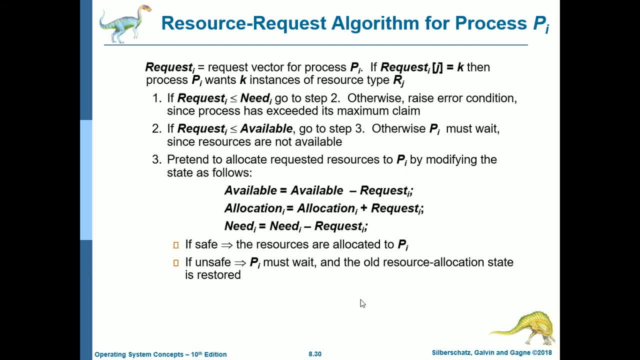 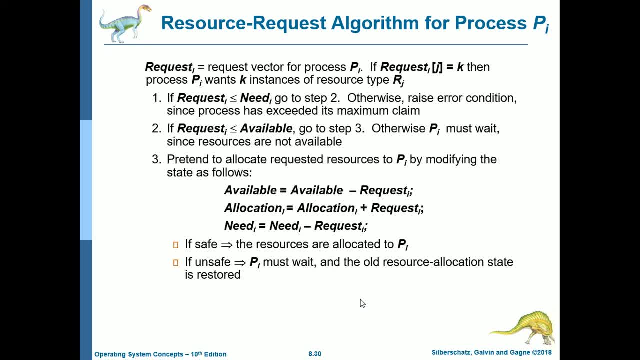 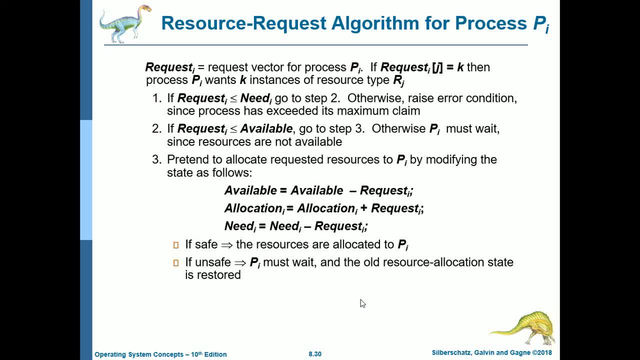 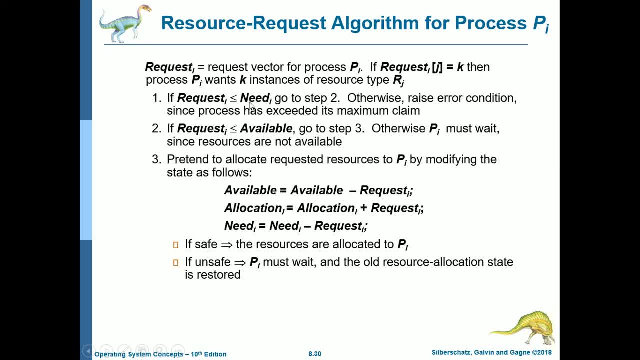 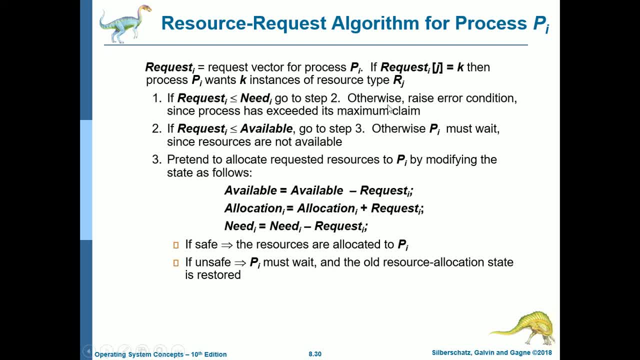 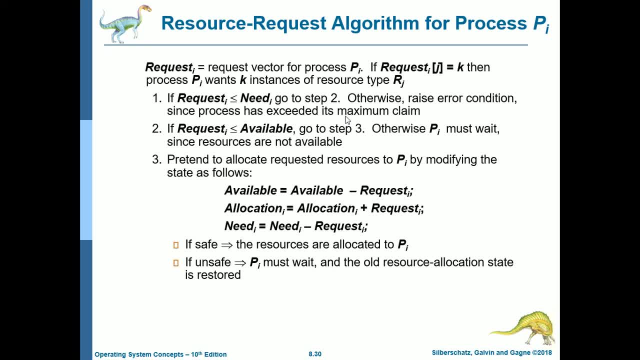 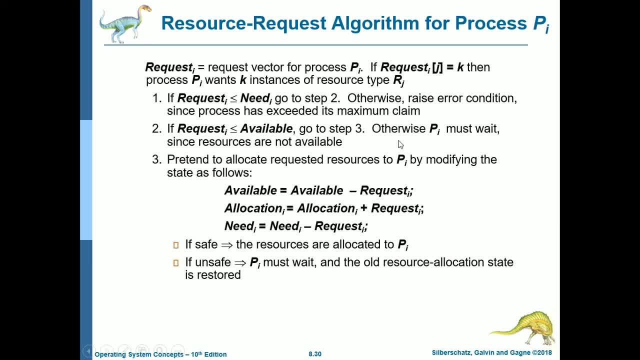 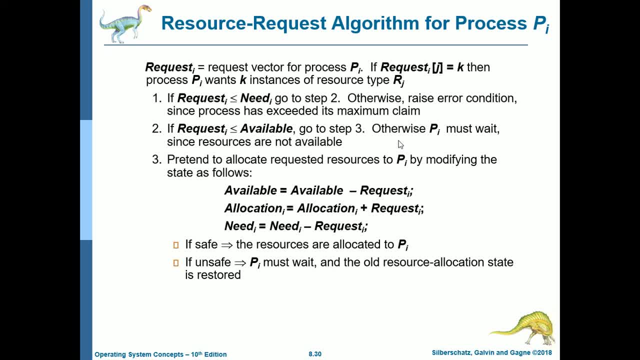 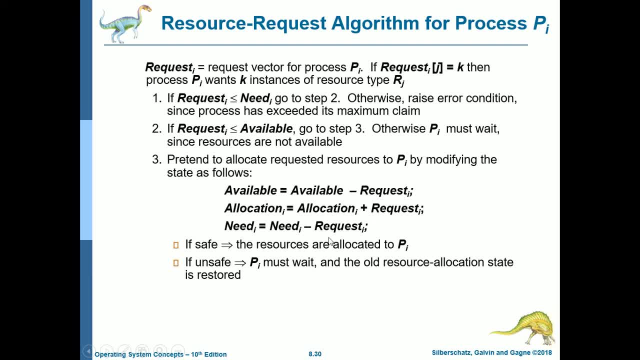 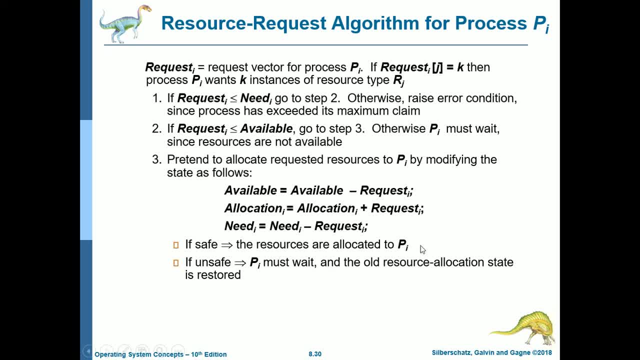 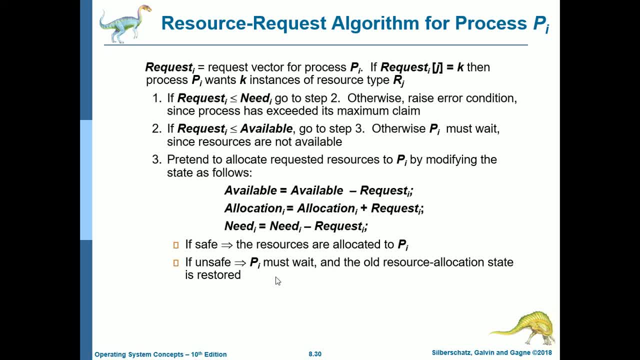 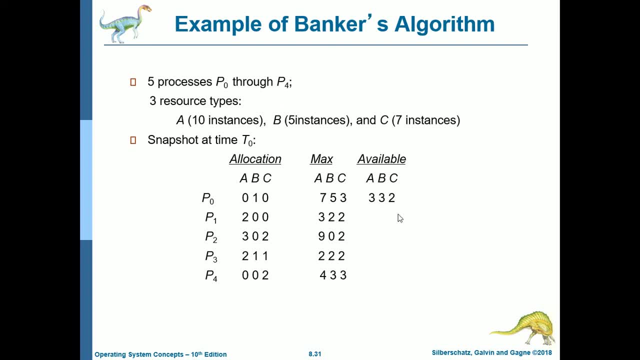 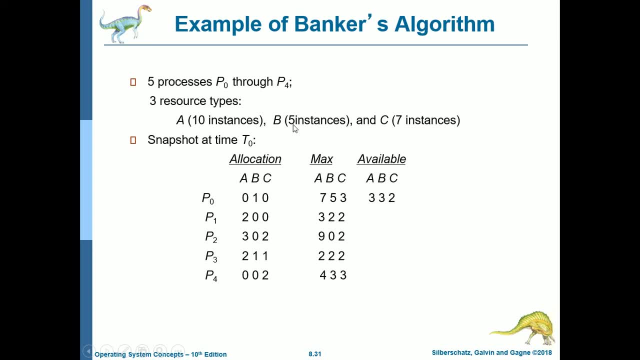 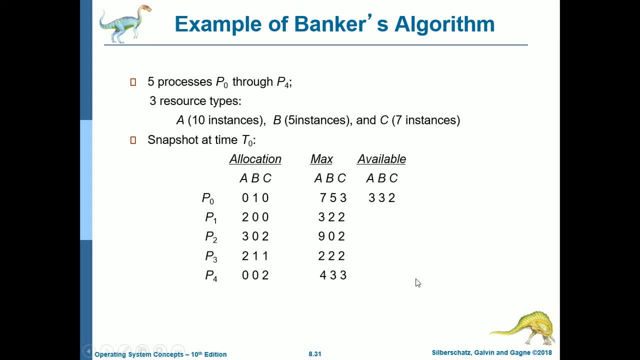 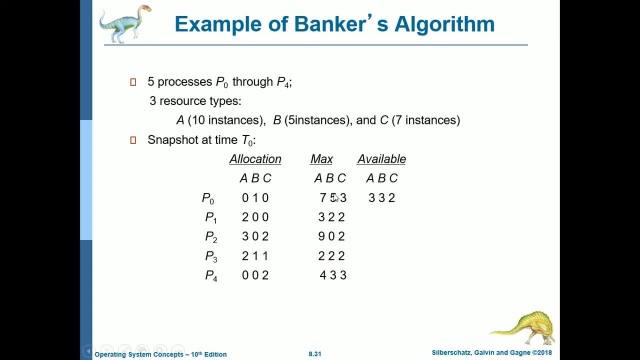 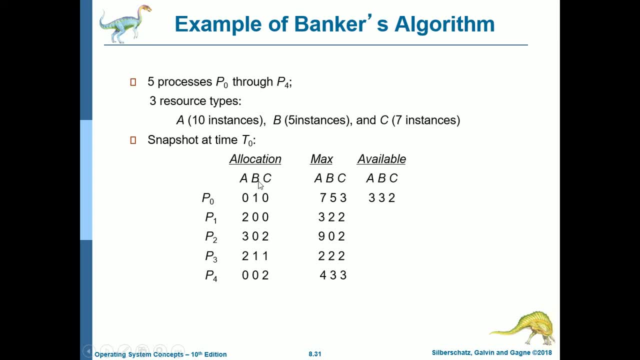 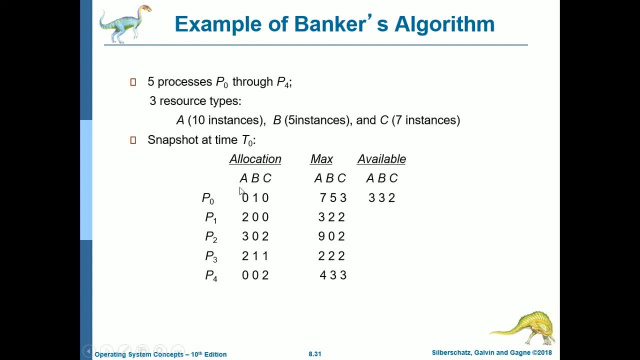 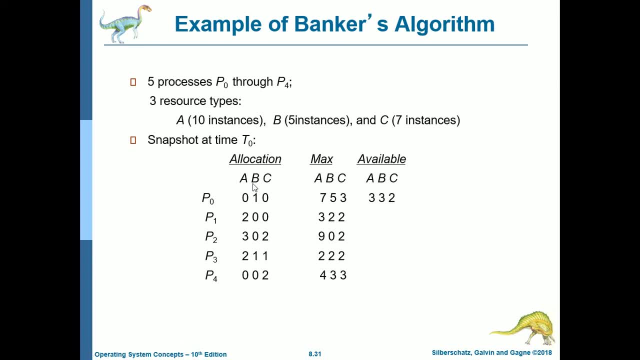 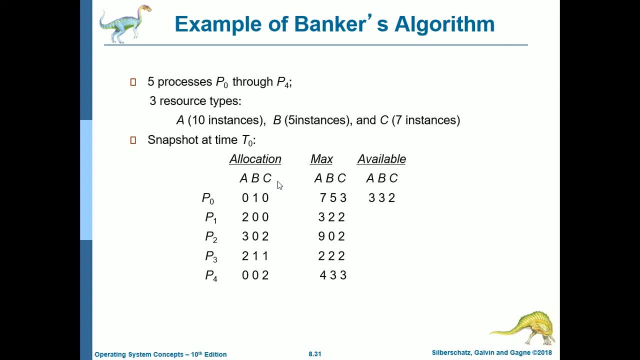 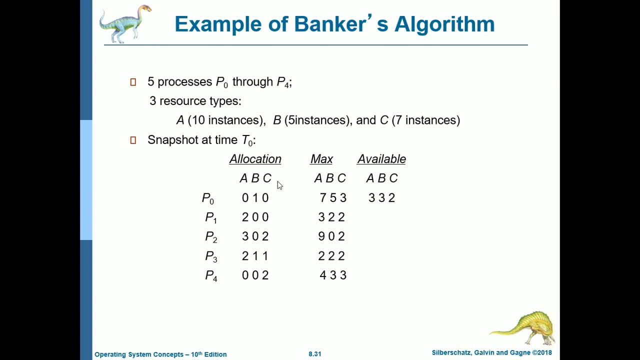 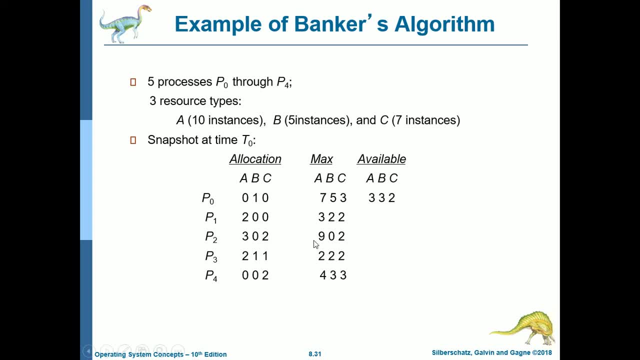 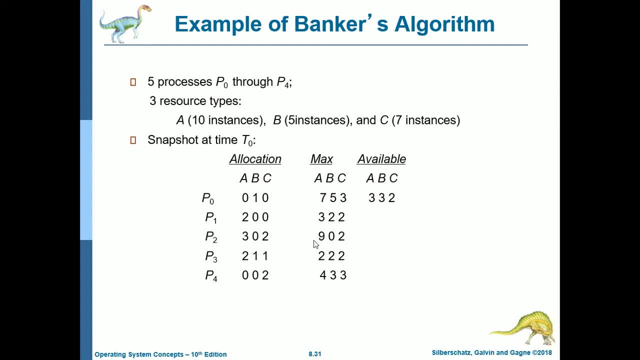 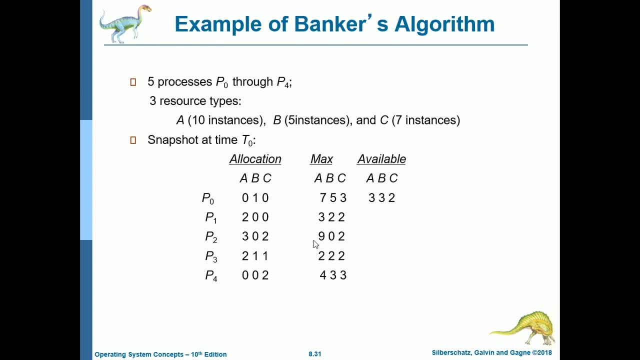 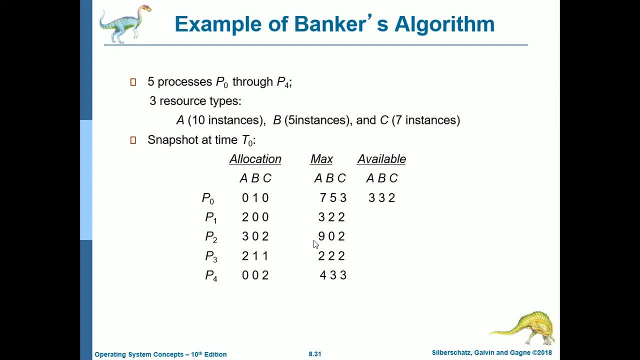 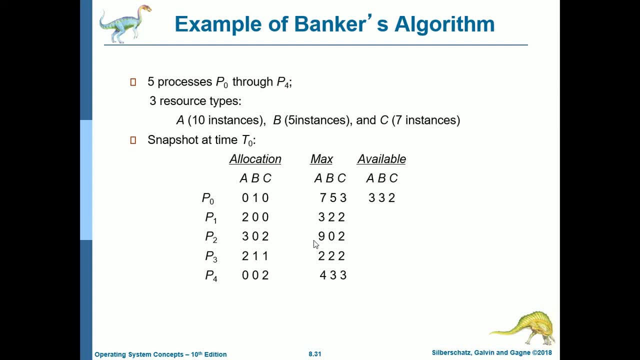 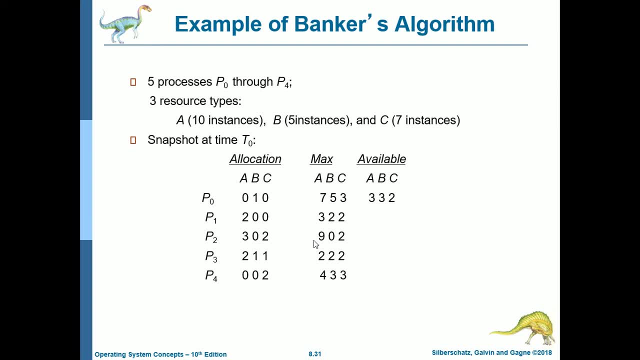 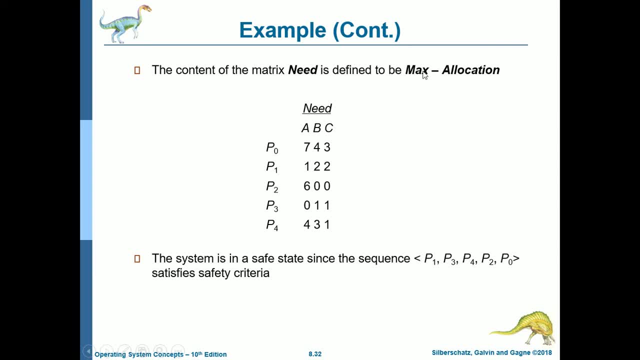 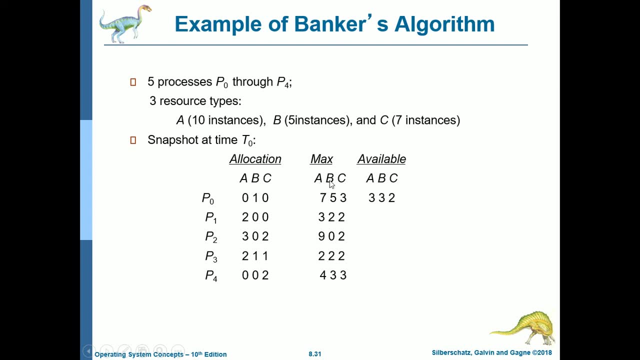 needed that particular resource, then it will be allocated to the processes that or threads that need, which is max minus allocation. so max minus allocation. so you're going to subtract from a to a, b to b, then c to c, and max, of course it should be max minus allocation after subtracting, uh, the. 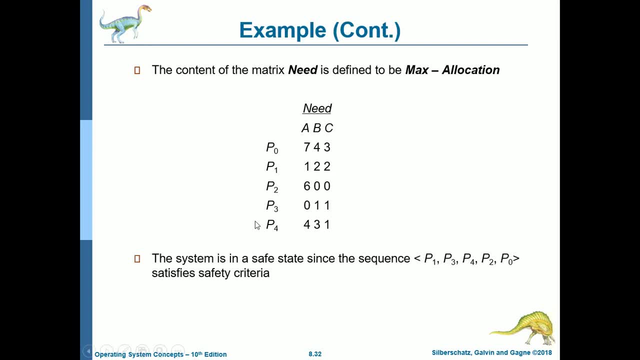 max minus allocation per process, is this is we, this is the result. so, by means of the need, so the system is in a safe state since the sequence. so we have this p, sub 1, p, sub 3 p, sub 4 p, sub 2 p. 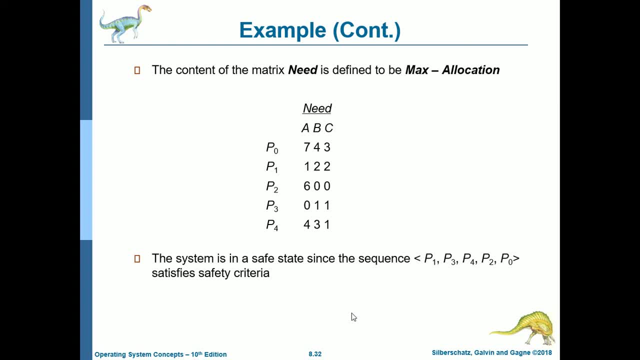 sub 0 satisfies safety criteria. so, again, i'm going to show you how thus this sequence happened. so why? why is the sequence like that? so, uh it, it is derived from from, of course, the banker's algorithm, from its algorithm. so, as you can remember, this is a system that is in a safe state since the sequence. so we have this: p sub 1, p sub 3, p sub 4. 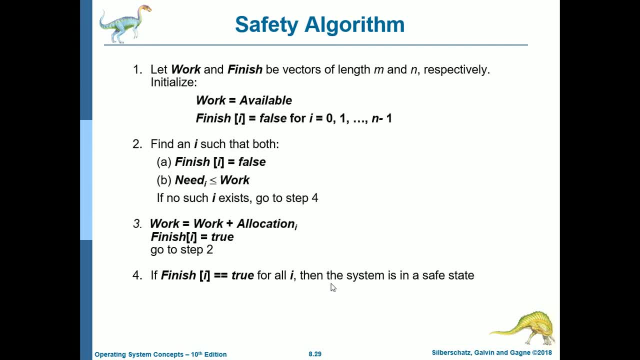 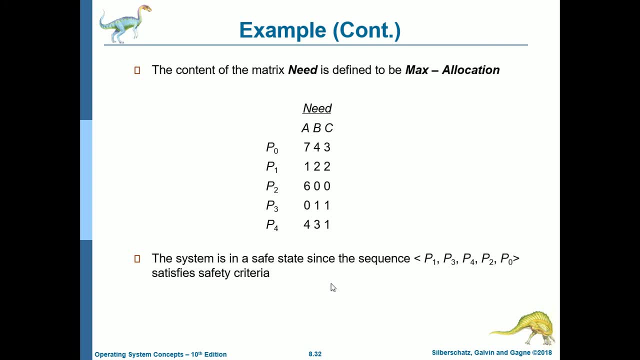 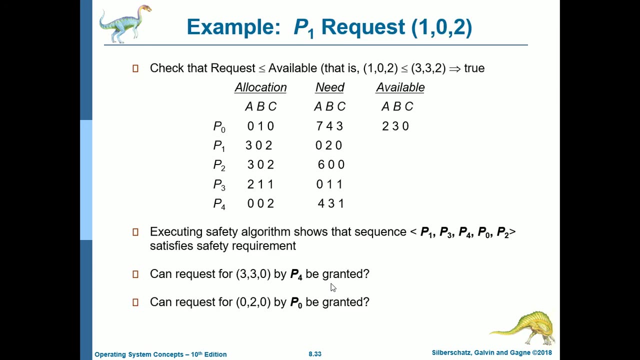 is the uh algorithm for that? okay, again, i'll provide a separate video for the illustration of the banker's algorithm that is given here in the slide presentation. so, uh, since for this example, so it is. it is in a safe state. what if p sub 1 requests for additional, additional resources? 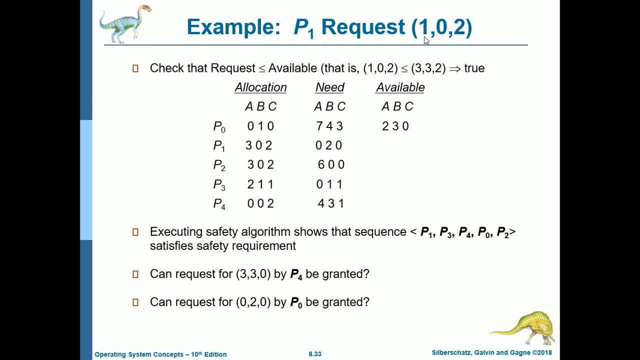 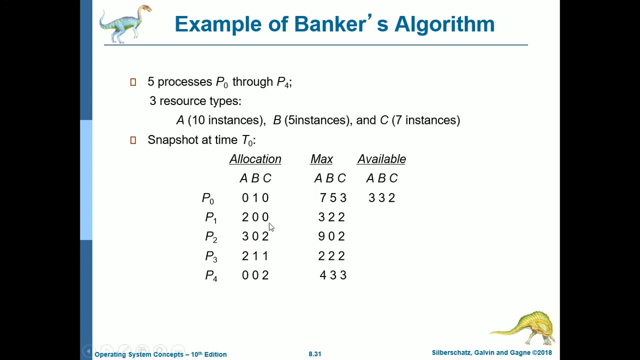 one resource type for for uh, one resource for uh, one resource for a, then it does not need any resource from b and two instances of resource c. so, as you can see what what happened. so what you what happened here is that, as you can see, p sub 1 is 2 0 0, since it requested uh plus 1 0 2. 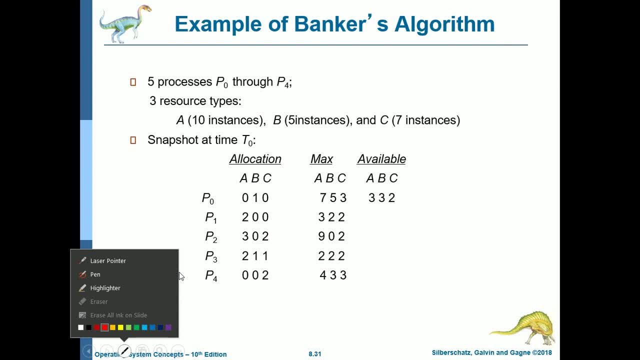 okay, since it has requested plus 1 0 2, you have, okay, okay, 1 0 2. you have to add that. so 1 plus 2 is equal to 3, then still 0, and then 2 plus 0 is equal to 2. so that's why the new allocated resource is 3 0 2. okay, but before you, 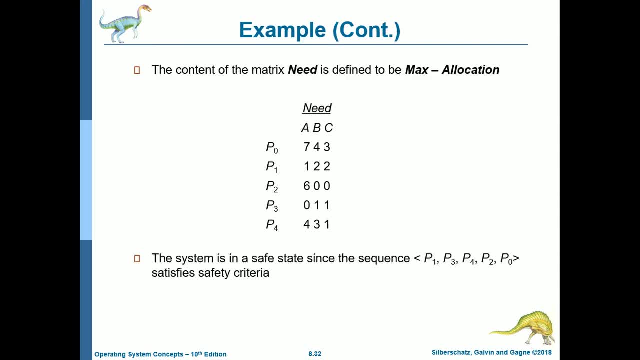 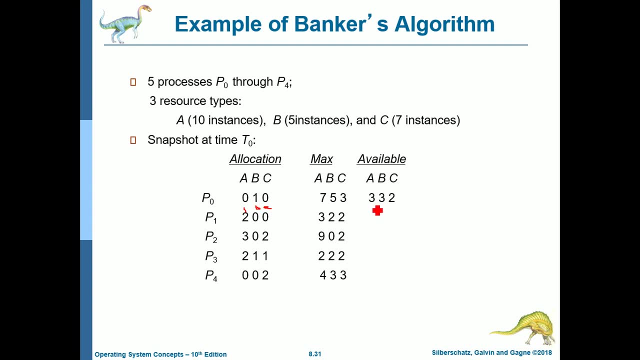 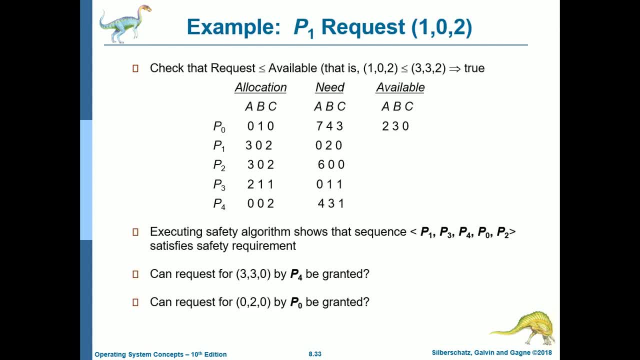 as you can see with our example here. so that's why this becomes 230. and then, after subtracting the request from the available, you have to add here in p, sub 1. so that's why it became 302. so check that request is less than or equal available. that is, so it is possible. so that's. 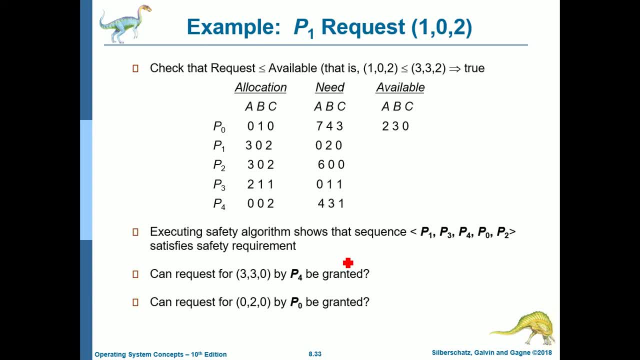 already subtracted, then executing safety algorithm shows that the sequence. so again by using again the banker's algorithm, so it satisfy the safety requirements. so the question now here if there is additional request for, for uh, for this a piece of four additional resources: a is three, b is three also, and 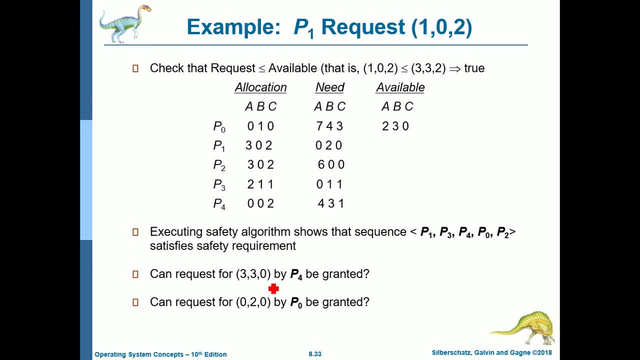 you can do that as well. so that's why we already subtracted. then executing safety algorithm shows does not need any resource from c. so, um, again, i'll provide this. um, actually, the answer here is it cannot be granted because there is not enough resource available, because 330 and you can already see here in the available. okay, of course, check for c, because it. 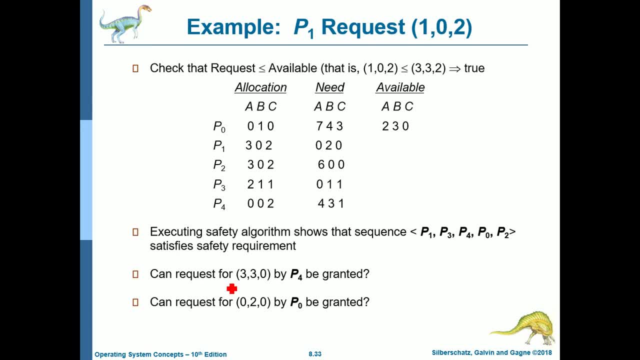 does not need any resources from c and b fits because the available resource is three. but the problem here is resource a, since the available is two- uh, this is already what- three, it exceeds the available. so, um, p4 requests for three instances of resource a and there's only two. 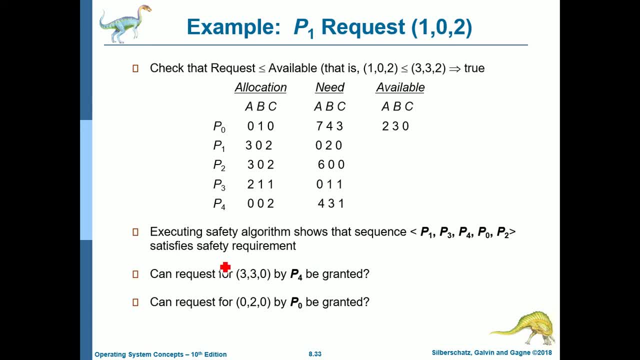 instance of resource a. so you, actually you can already answer, but uh, again, i also provided in in the uh additional video for this one. so another question is: can request for zero to zero by p sub zero be granted? so we're going to have zero to zero, so, but but before that. so this is: 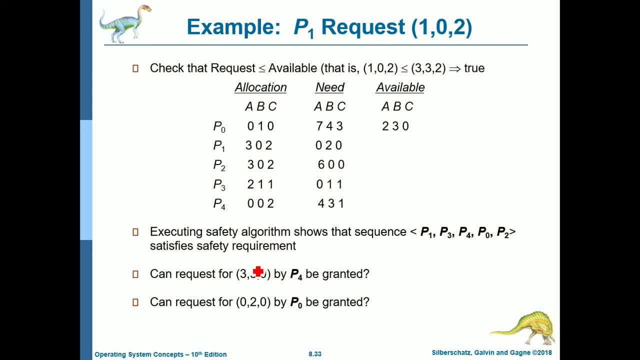 already the piece of one is already requested. one zero, two, so actually, um, it still fits. so we're going to subtract, so zero, two, zero, so subtract, so we have zero one, two. this is the available resource, so it's still less than the available, so the request, so 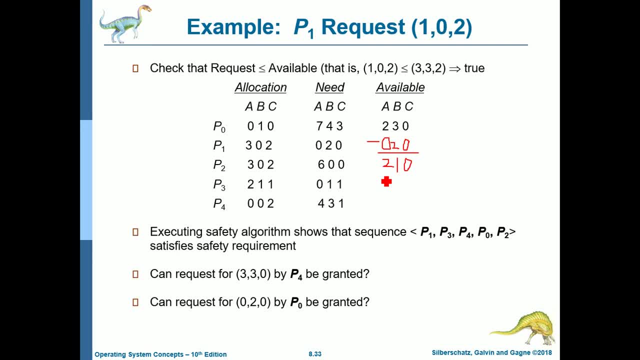 but the answer is this: if you're going to again use the banker's algorithm, the answer will be: though the resource is requested by p, sub zero can be granted because it fits the uh available, a, b and c okay, but the system is in unsafe state because there is no sequence of the processes. 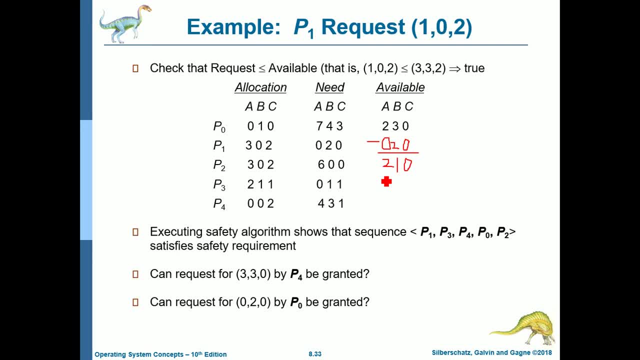 that satisfies the safety criteria. if you're going to use the banker's algorithm, you cannot produce a sequence that satisfies the safety criteria. you can only allocate the resource for p sub zero, but you cannot continue its process because it is already unsafe. so, again, i'll provide an additional video so that you can see why. uh. 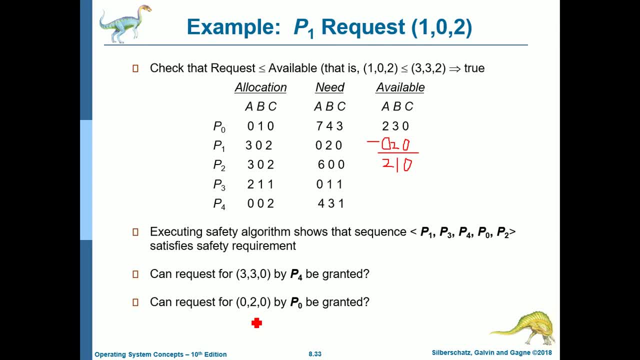 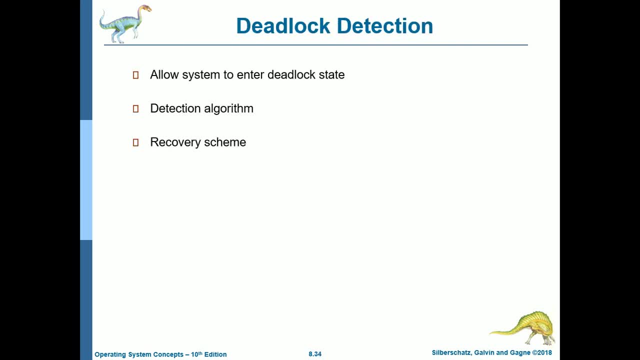 why uh requesting uh, additional, uh, additional resources from p sub zero will leave the system in unsafe state. okay, next is we have the deadlock detection, so allow system to enter deadlocked. and then we also have the detection algorithm and recovery skin. so for the single instance of 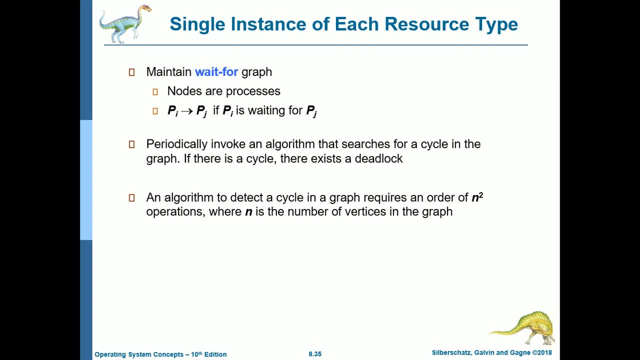 each resource type. so we have this. maintain weight per graph. so nodes are processes for p sub i to p sub j. if p sub i is waiting for p sub j periodically, invoke an algorithm that searches for a cycle in the graph. if there is a cycle, there exists a deadlock, of course. 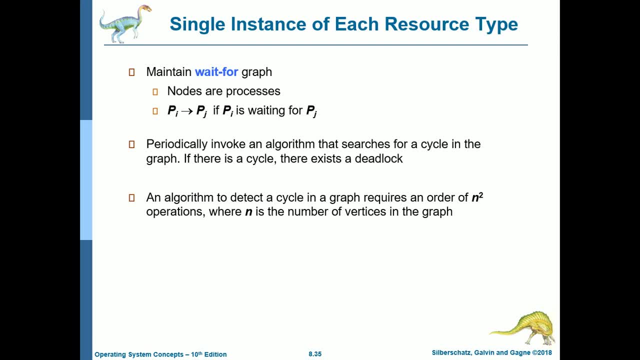 and then an algorithm to detect a cycle in a graph requires an order of n squared operations, where n is the number of vertices in the graph. so a cycle, if all the processes are involved, that is the what holds true for deadlock to occur. okay, so this is the comparison between a resource. 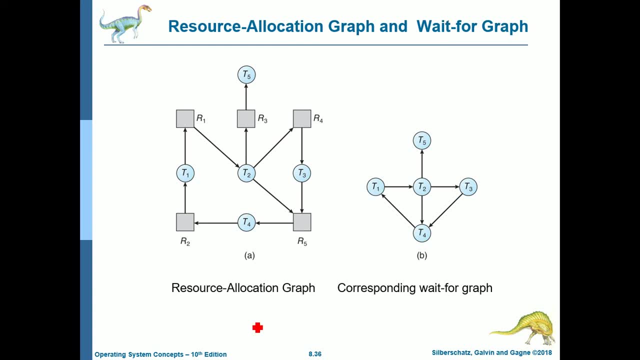 allocation graph and the weight for graph. so this is the resource allocation graph, so we have the resources. so the only difference for the weight for graph is you have to remove the resources and redirect the arrows. so, for example, t sub 1. t sub 1 needs a resource r sub 1 that is held by t sub 2. 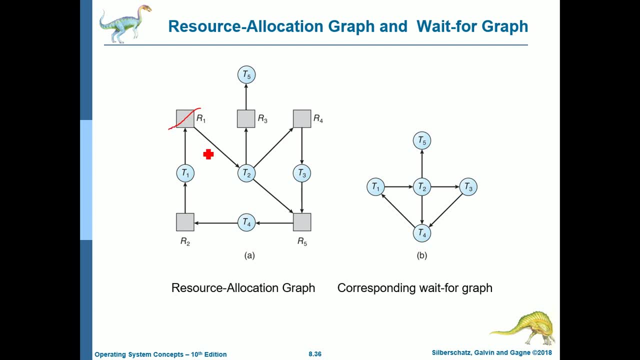 so just remove r sub 1 and then, since r sub 1 is assigned to t sub 2, then connect t sub 1 to t sub 2 and then another one, t sub 2. so this is already okay. t sub 2 needs a resource that is held. 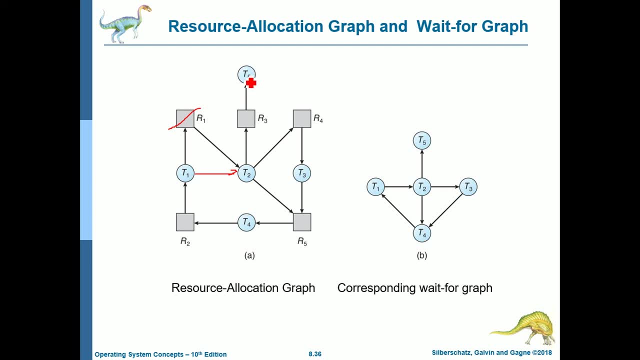 resource 3 that is held by by t sub 5, so let's just redirect it. and then next is we have t sub 3, so t sub t sub 2 also, so t sub 2 needs a resource. resource 4 that is held by t sub 3, so just remove resource uh 4 and 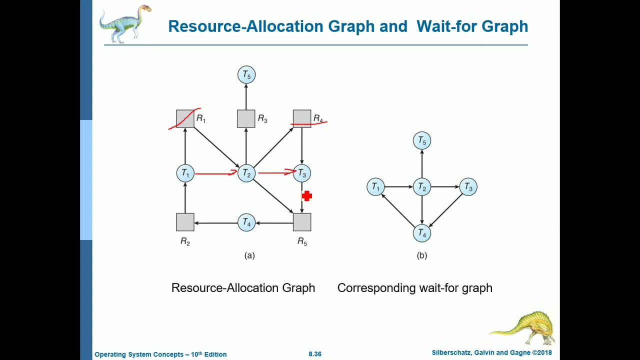 then redirect it to t sub 3, and then t sub 3 needs a resource that is held by t sub 4, so we have this one, and then t sub 4 needs a resource that is held by t sub 1. so, okay, just remove the resources. so this is the weight for graph. okay, then also t sub 2. 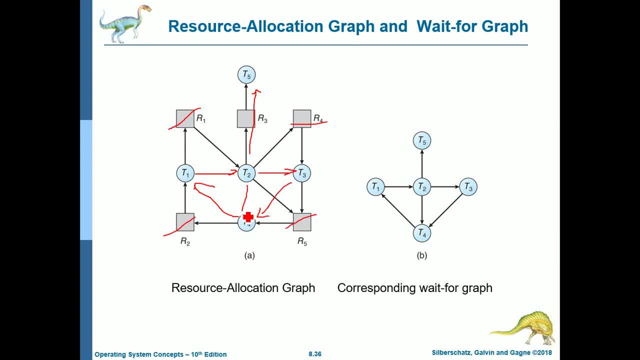 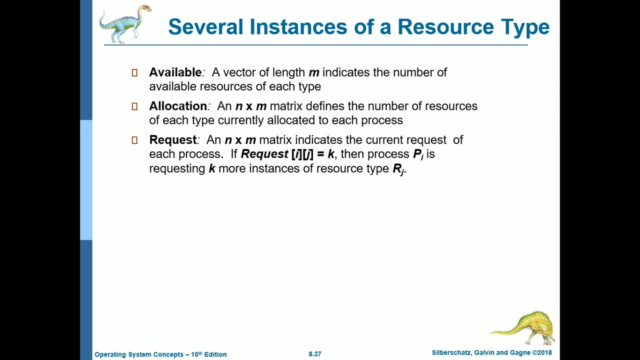 needs a resource that is held by t sub 4. so that is the weight for graph. you can derive a weight for graph corresponding to its resource allocation graph. okay, next is what we have. what is? we have several instances of a resource type so available. a vector of length m indicates the number of available resources of each type. 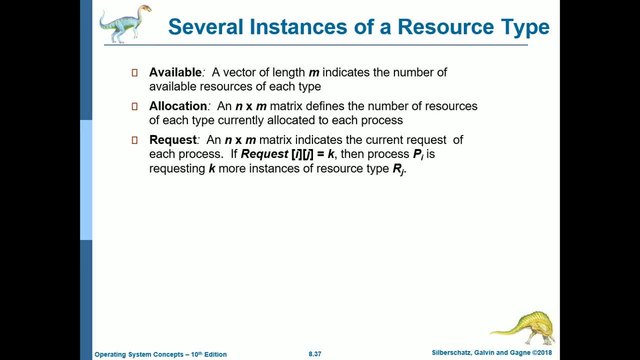 and allocation is n by m. matrix defines the number of resources of each type currently allocated to each process, and then request is n by m. matrix indicates the current request of each process. if request i, j is equal to k, then process p, sub i is requesting k. 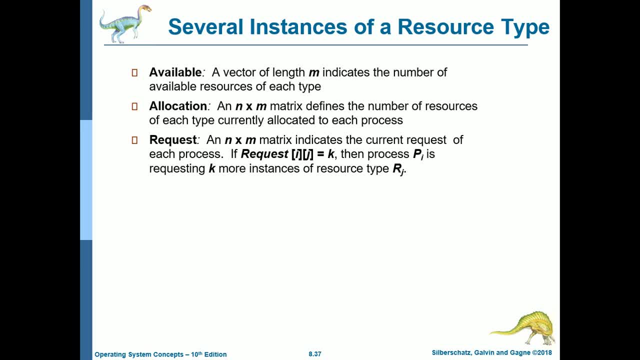 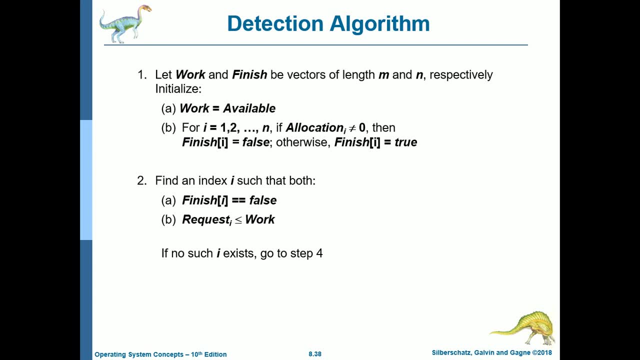 more instances of resource type rj. so the detection algorithm. so let work. and finish. be vectors of length, m and m respectively. so initialize: work is equals available for i is equal to 1 to n. if allocation is not allocation, sub i is not equal to 0, then 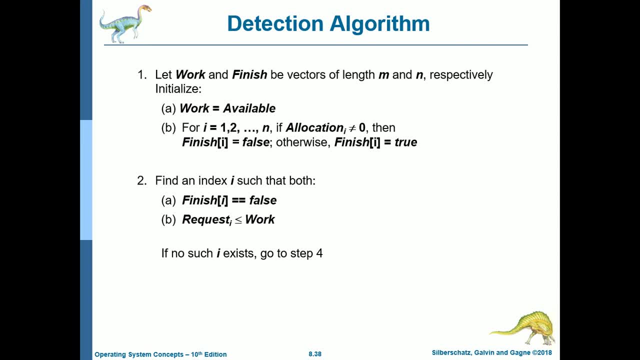 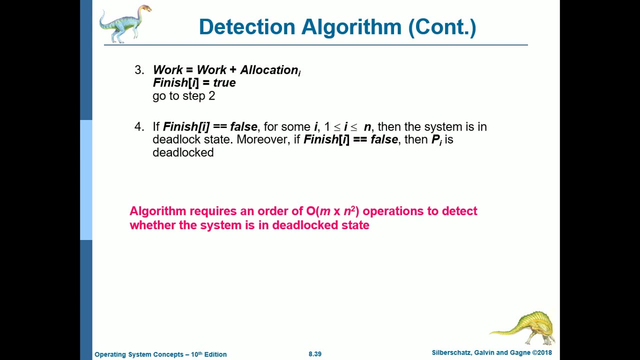 finish is equal to false, otherwise finish is equal to true. find an index i such that both is finished is equivalent to false, and request sub i is less than or equal to work. if no such i exists, go to step four. so for step three is work is equal. 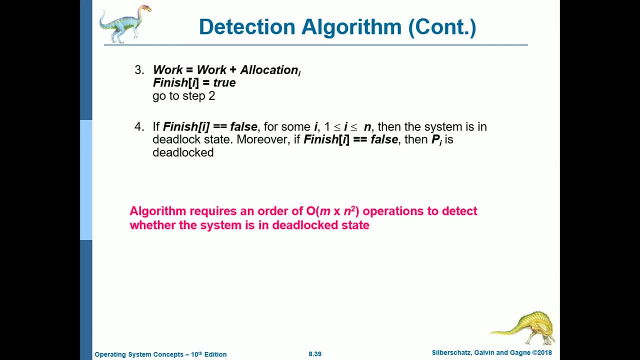 to work plus allocation, finish is equal. to then go to step two. actually, detection algorithm is similar to banker's algorithm. the only difference is that you can see in our example. i'll show you the difference between banker's algorithm and detection algorithm, but their their way of. 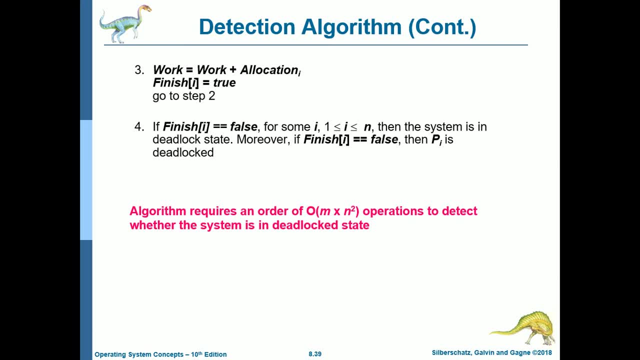 using resources and returning all the resources, that the process or the threads is used. it's just the same with banker's algorithm. so next step four, finish, is equivalent to false for some i i is less than or equal to. i is less than equal to n, then the system is in a deadlock state. moreover, if 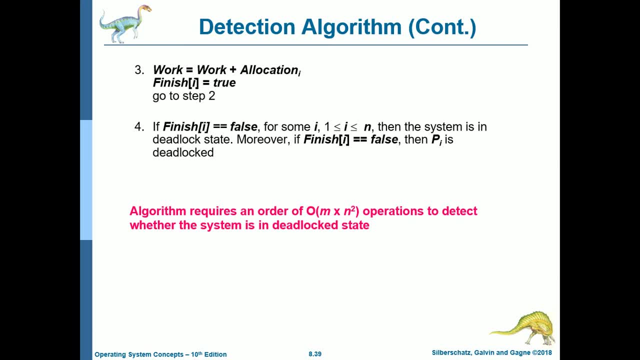 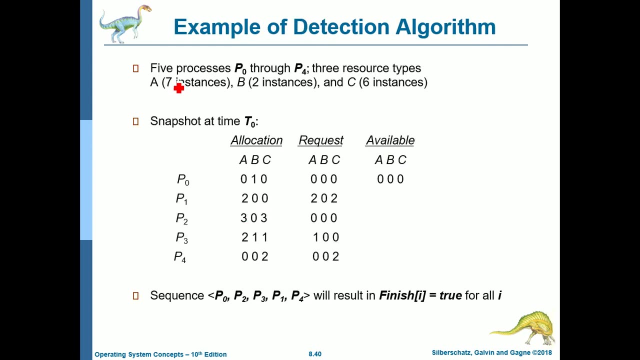 finish is equivalent to false, then p sub i is deadlocked. so this algorithm requires an order of o m times n squared operations to detect whether the system is in a deadlocked state or not. system is in a deadlock state. okay, this is an example of detection algorithm. so five processes. 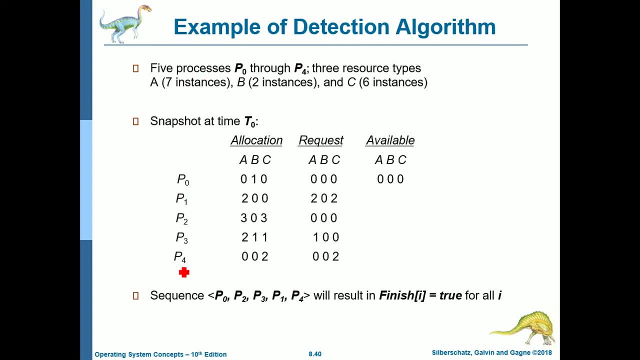 again from p sub zero to p sub four, then three resource types. so a has seven instances, b is a total of two instances and c has a total of six instances. so this is the snapshot, so the difference between banker's algorithm. so they have the same allocation, matrix, matrix and available vector. 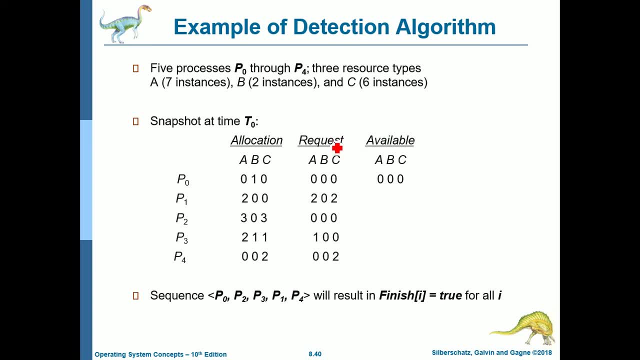 the only difference is that for uh banker's algorithm, uh the given, the given in a banker's algorithm is the max matrix, while for the detection algorithm is. we have request so for this snapshot. so sequence p sub 0, p sub 2, p sub 3, p sub 1 and p sub 4 will result in finish. i is equal, true for all. 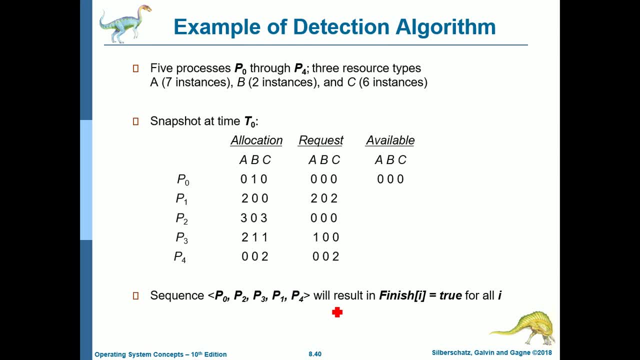 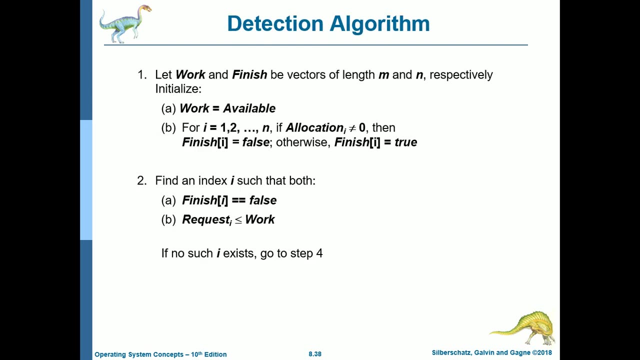 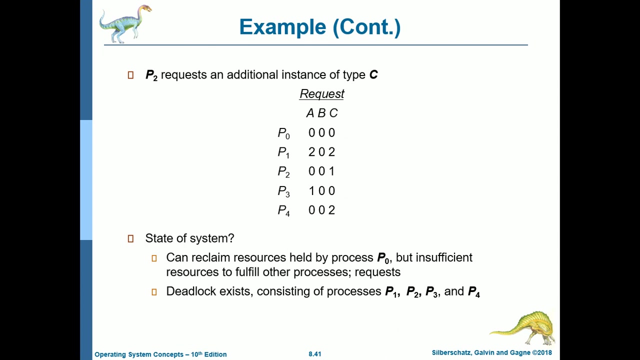 i again, i'm going to provide an additional video for you to see. how does this sequence, uh, how, why is this the sequence like this? it's, uh, of course it's by using again the detection algorithm that is stated in here for you to better understand. okay, next, what if p, sub 2 request an additional resource of? 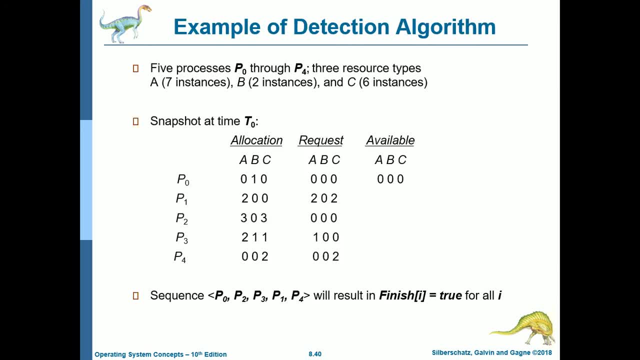 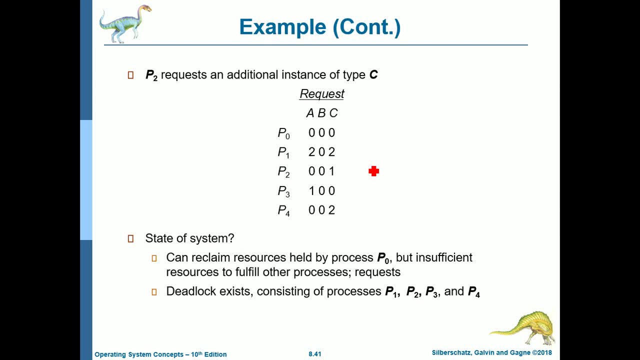 type c. so previously the request does not have any requests for any of the resources, but now it requests for an additional instance of type c. so that's why p sub 2 becomes zero, zero one. so what is the state of the system? so actually can reclaim resources held by process, piece of zero but insufficient resources to 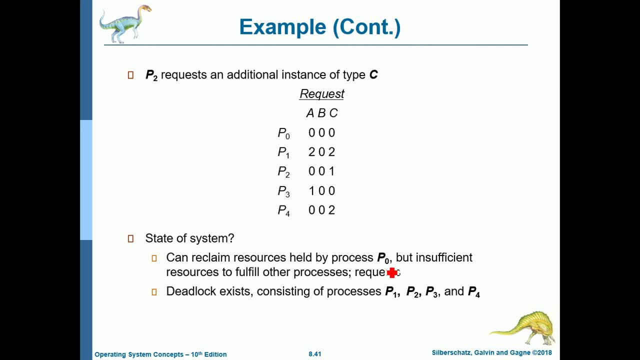 fulfill other processes or requests. so since uh it only executed p sub zero, it only finished its execution and then the next, the next um processes did not continue its execution. so deadlock exists, consisting of processes p sub 1, p sub 2, p sub 3 and p sub 4. again, i'm going to show you. 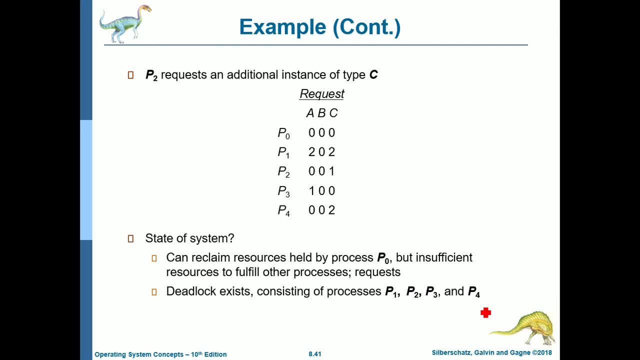 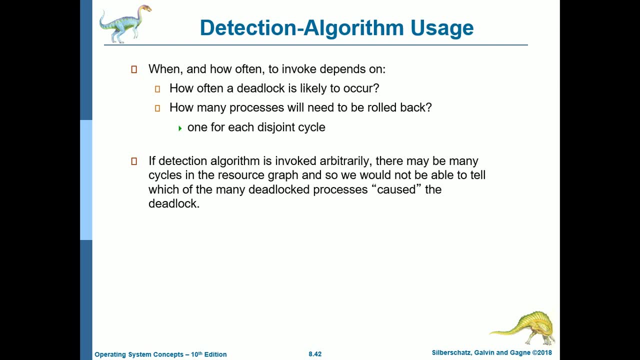 uh, how does this happen? by an additional video? okay, we have detection algorithm usage. when and how often to invoke depends on how often a deadlock is likely to occur and how many processes will be executed. relationship regional: we want to introduce a process check that makes sure that each process is 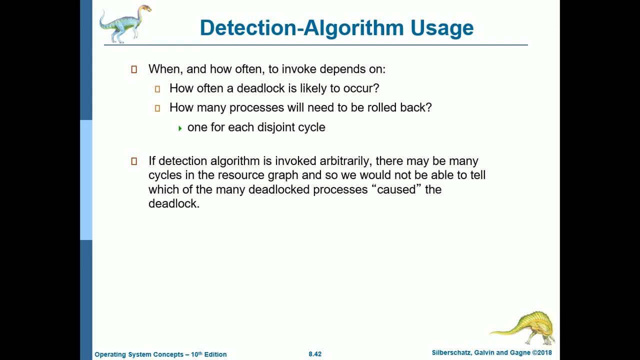 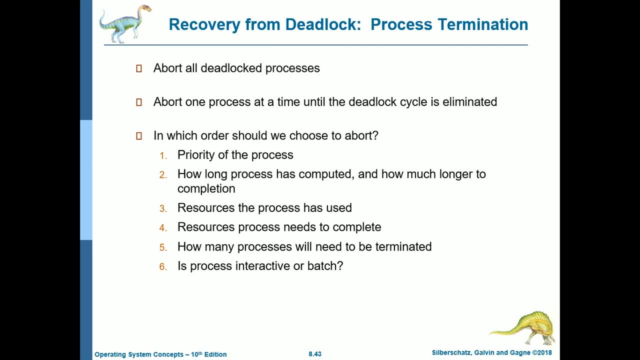 machine starts discussed and they will come up with a result. so how is the process counted and what will it mean? well, here we can. you can use this process termination to filter workers toowan. so early on in the does it be implemented in the computer system. so abort all deadlock processes or abort one process. 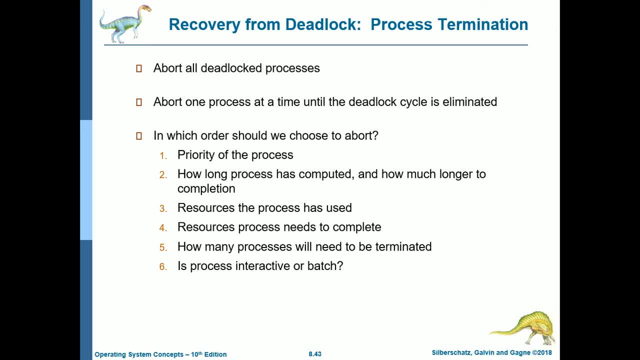 at a time until the deadlock cycle is eliminated. in which order should we choose to abort? first is the priority of the process- how long process is computed and how much longer to completion- and resources the process is used. resources that the process needs to complete: how many processes. 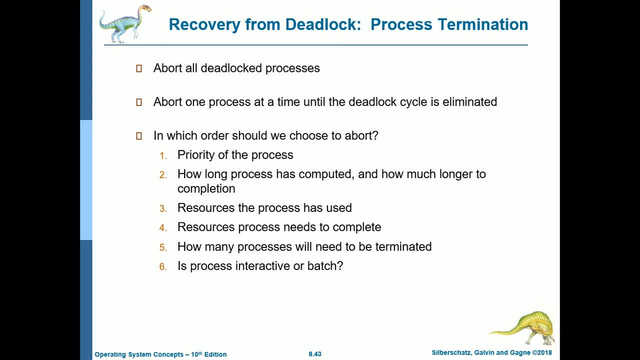 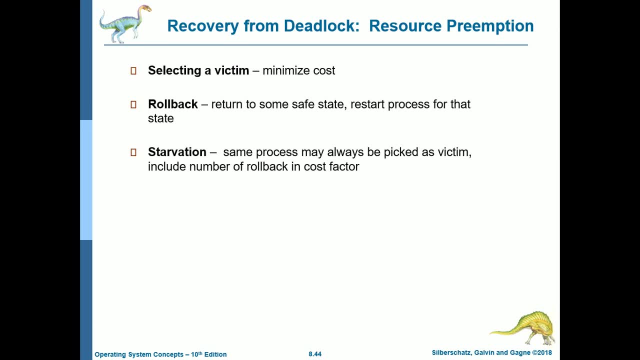 will need to be terminated. and is the process interactive or batch? okay? another one is resource preemption, so you have to select a victim. this is to minimize the cost or rollback, return to some safe state, restart process for that state and starvation- same process may always be picked. 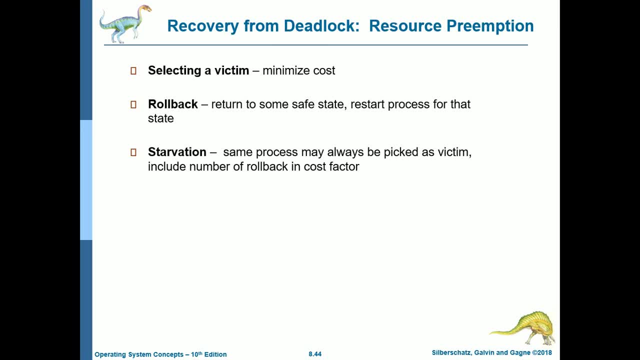 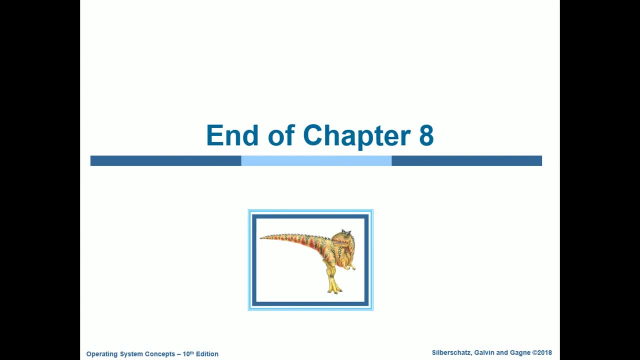 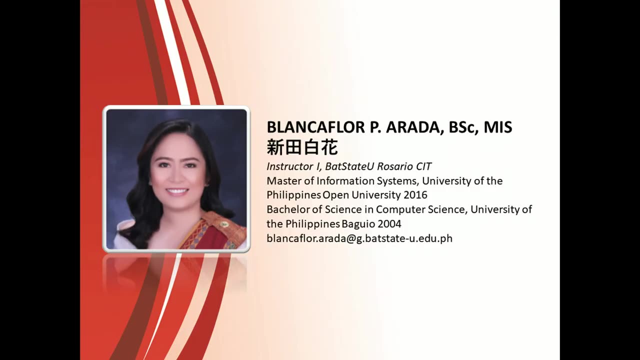 as victim, include number of rollback in cost factor. so this is already the waste. on how to avoid deadlocks. so we have a banker's algorithm and detection, deadlock detection algorithm. so, again, i will provide additional video for you to illustrate. how does this sequence, how does this sequence produced? so if you do have any questions, so please feel free to comment.